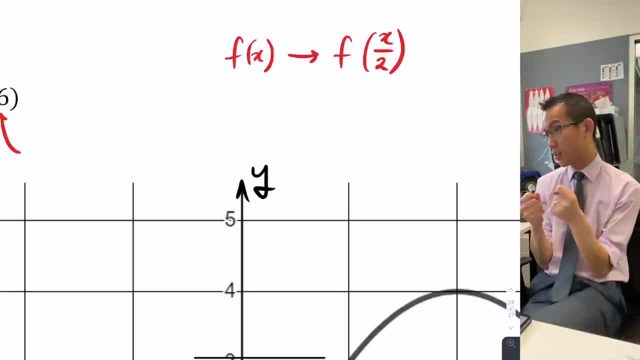 What it would look like is the same graph, but it's been dilated or stretched out. It's twice as wide, so it looks like it's gained some weight. And it's wide because what's being changed here is the x, And x is horizontal. 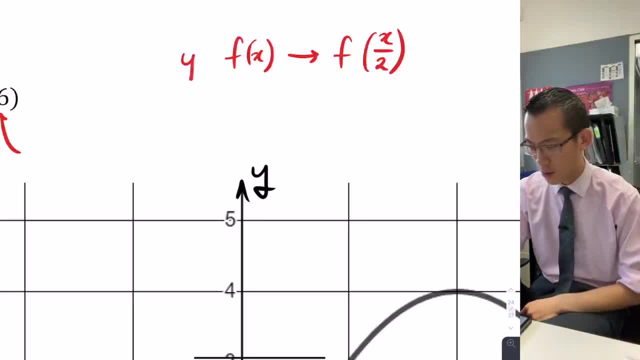 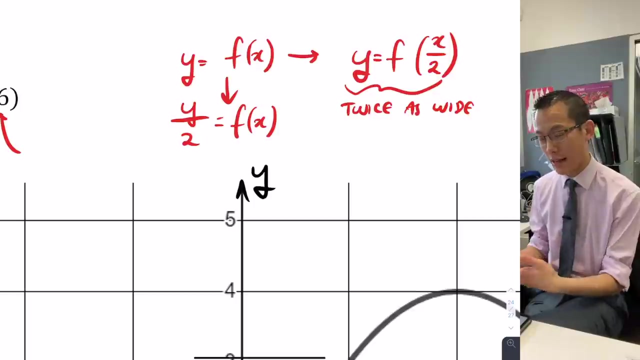 Does that make sense? So if, by contrast, like say that was y equals f, like that, so I'll put a y equals over here, This guy is twice as wide. Now, if I said instead of x on 2,, if I said y on 2, again, this is another dilation, because 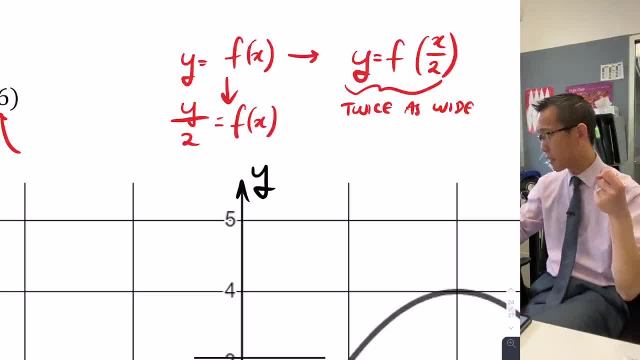 it's a multiplication or division, but it's not going to be wider because I'm not changing x anymore, I'm changing y. So instead of being bigger this way, yeah, you're going to stretch vertically, Exactly, right? So this, I guess you'd say it's twice as tall, right? 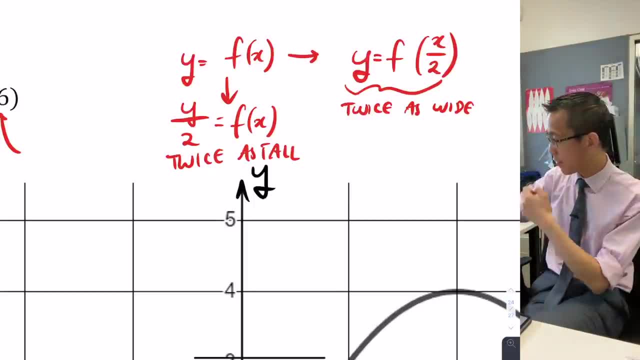 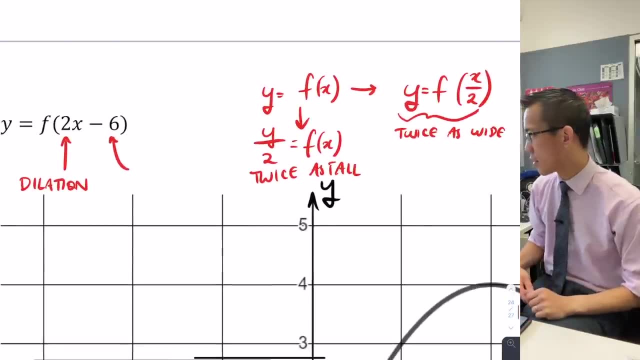 So this is what happens when you make things bigger: if you're doing it vertically or if you're doing it horizontally. Now, if you have a look over here, what I've got here is not x divided by 2.. I have x multiplied by 2, yeah. 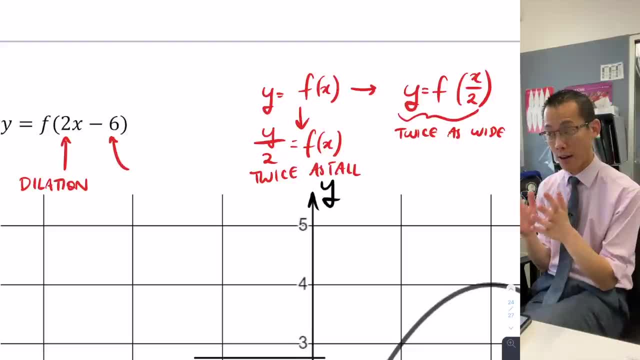 So you know how I said that these ones over on the right-hand side, they make things taller or wider. Yeah, Yeah, this is going to get squashed in, so it's going to get compressed. So because it's a 2 there, I'm going to say this is sort of, yeah, compressed. 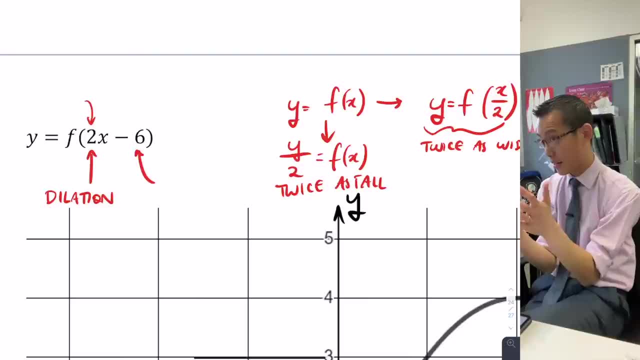 It's everything that used to take up this amount of space is now taking up half that space, okay, Which is a bit weird. It's a bit reversed, okay, But yeah, I think that's an okay thing to say. So let's write in that this is going to be half the width, I guess is a way to say it. 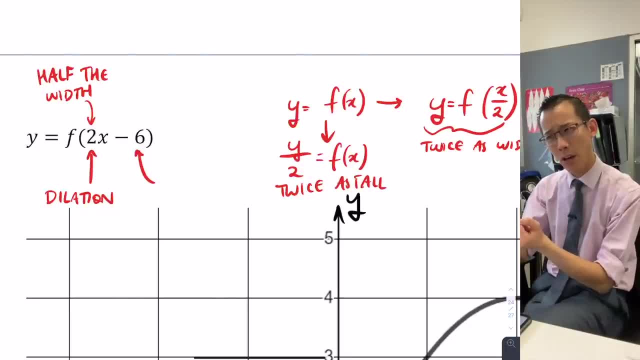 Can you remind me as well? how did I know that it's width and not height that's being changed? It's the f of x. Very good, Yeah, In relation to x, not y. Yeah, exactly, So you can see. the change is happening on this pronumeral, not the other one, okay. 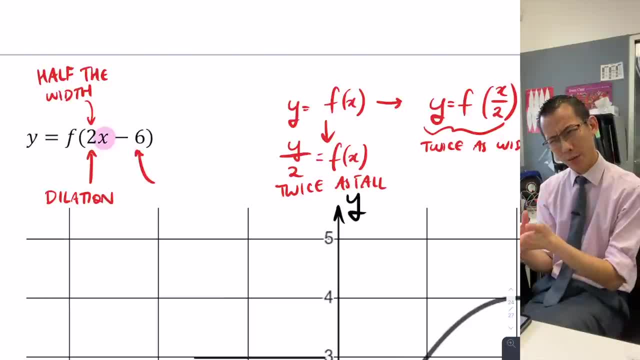 Very good, Okay, very good. So I've got that, And then I've got to deal with this minus 6.. So this is not a dilation, this is what we call a translation. So it's where it moves. Yeah, exactly. 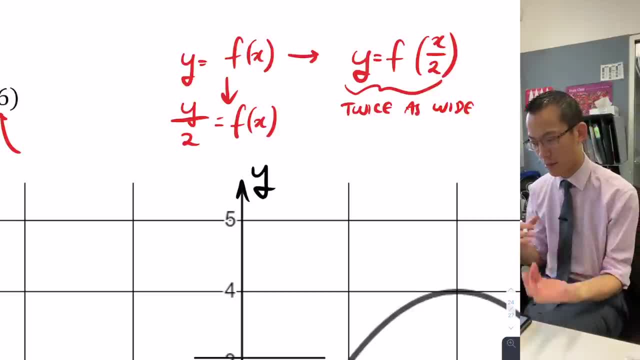 again, this is another dilation, because it's a multiplication or division, but it's not going to be wider because I'm not changing x anymore, I'm changing y. So instead of being bigger this way, yeah, you're going to stretch vertically. 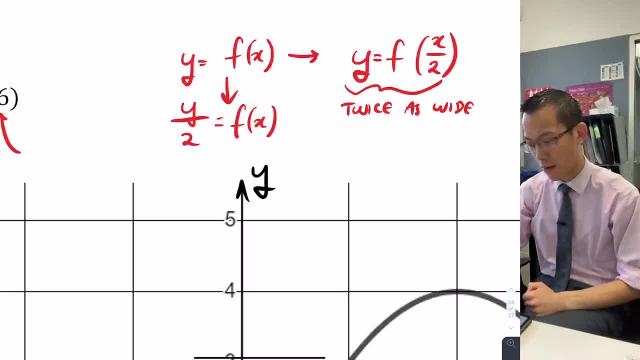 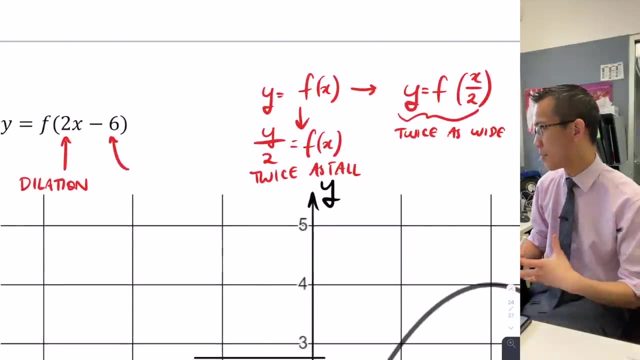 Exactly right, Because I guess you'd say it's twice as tall, right? So this is what happens when you make things bigger: if you're doing it vertically or if you're doing it horizontally. Now, if you have a look over here, what I've got here is not x divided by 2.. 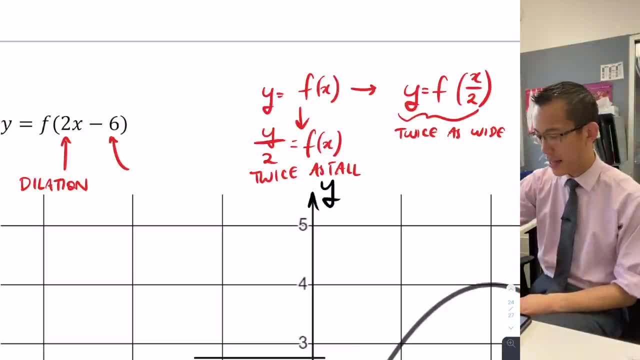 I have x multiplied by 2, yeah, So you know how I said that these ones over on the right-hand side they make things taller or wider. Yeah, this is going to get squashed in, so it's going to get compressed. 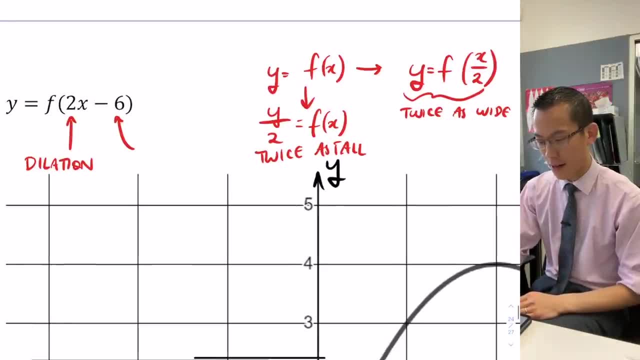 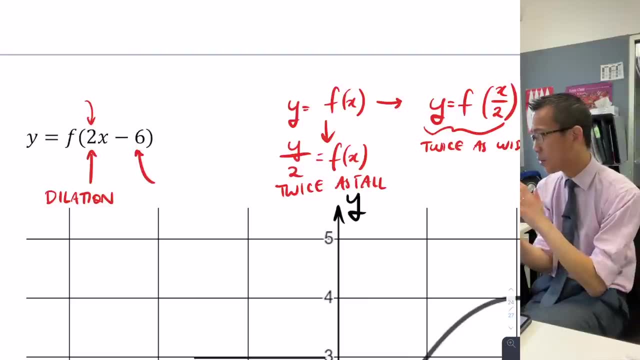 So, because it's a 2 there, I'm going to say this is sort of: yeah, compressed, It's everything that used to take up this amount of space is now taking up half that space, okay, Which is a bit weird. 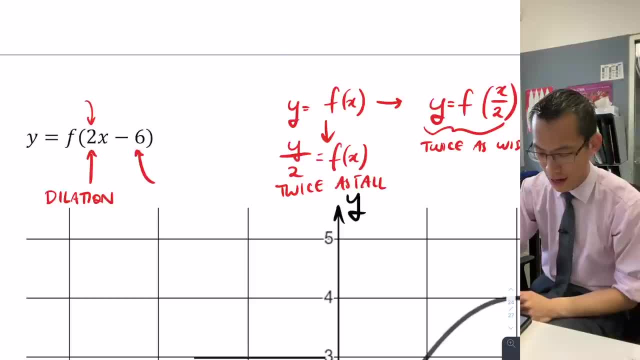 It's a bit reversed, okay, But yeah, I think that's an okay thing to say. So let's write in that this is going to be half the width, I guess is a way to say it. Can you remind me as well? 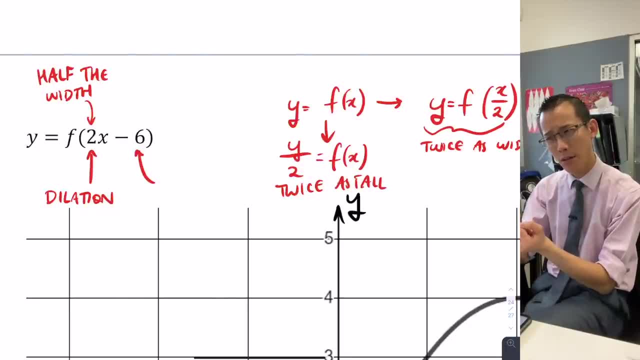 how did I know that it's width and not height that's being changed. It's the f of x. Very good, yeah, In relation to x, not y. Yeah, exactly, So you can see the change is happening on this pronumeral. 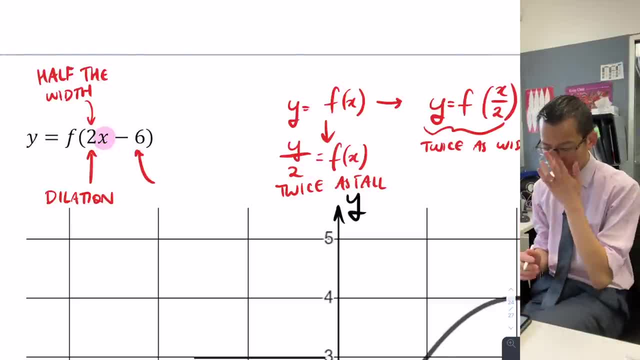 not the other one. Okay, very good. Okay, very good. So I've got that, And then I've got to deal with this minus 6.. So this is not a dilation, This is what we call a translation. So it's where it moves. 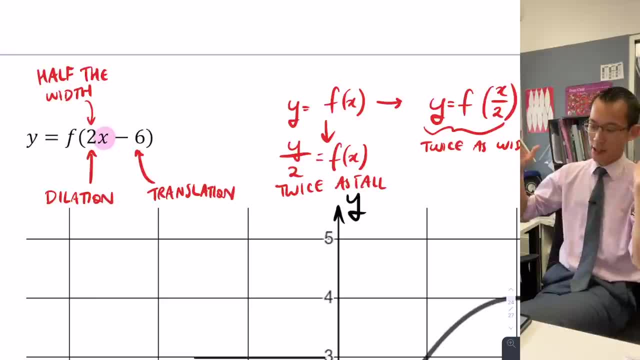 Yeah, exactly, So we actually met this word all the way back in U7, which was a long time ago. It's about taking the shape and then, like the synonym we used to use was we slide it around or we shift it around? okay, 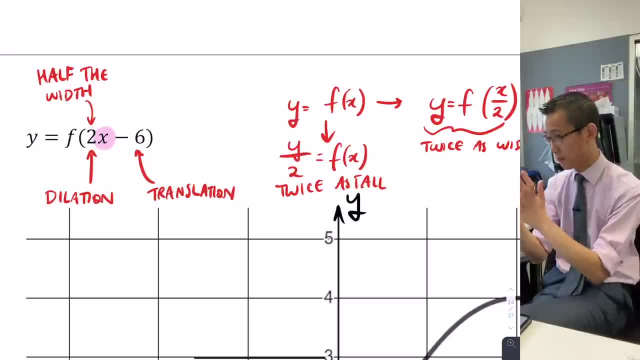 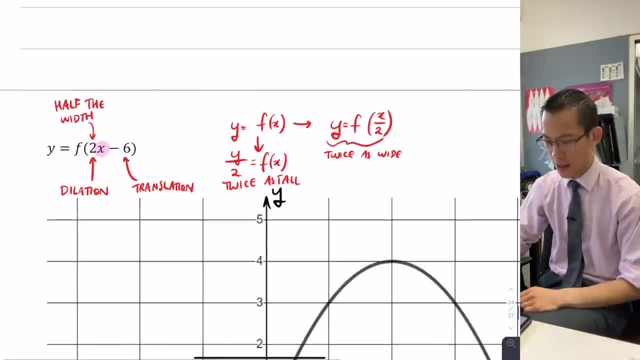 So once we've worked out how big it is, we then say, okay, what position is it in? Okay, Now there's kind of a sneaky thing here and we've got – let's actually use the space underneath the graph. 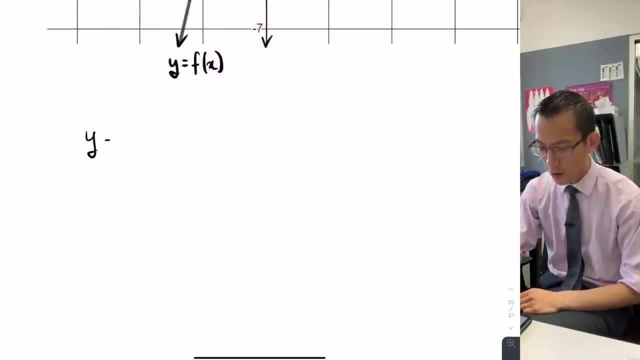 because we've got some space down there. You've been given y equals f of 2x minus 6, like so, And we said, oh okay, it's going to be half the width, so we will work out what that looks like in a second. 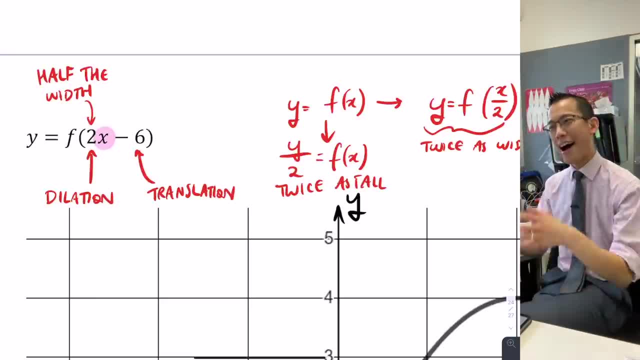 So we actually met this word all the way back in Year 7, which was a long time ago. It's about taking the shape and then, like the synonym we used to use was we slide it around, We lift it around, okay. So once we've worked out how big it is, we then say, okay, what position is it in? okay, 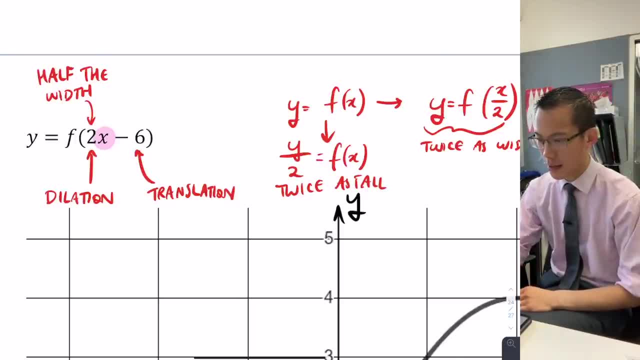 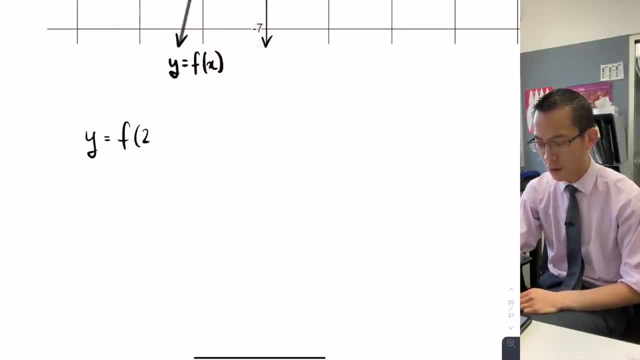 Now there's kind of a sneaky thing here and we've got- let's actually use the space underneath the graph, because we've got some space down there. You've been given: y equals f of 2x minus 6, like so. 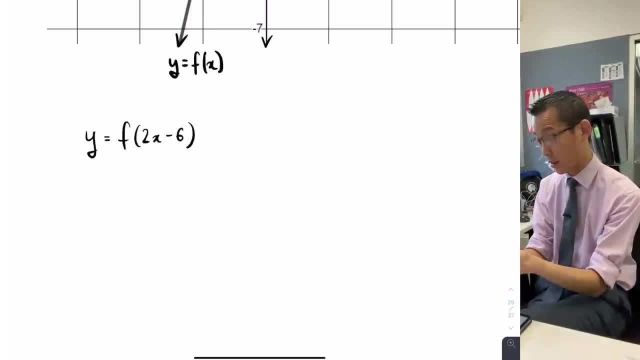 And we said, oh, okay, it's going to be half the width, so we will work out what that looks like in a second. but that minus 6, it sort of seems like, okay, you're going to move, you're going to move 6 units, right. 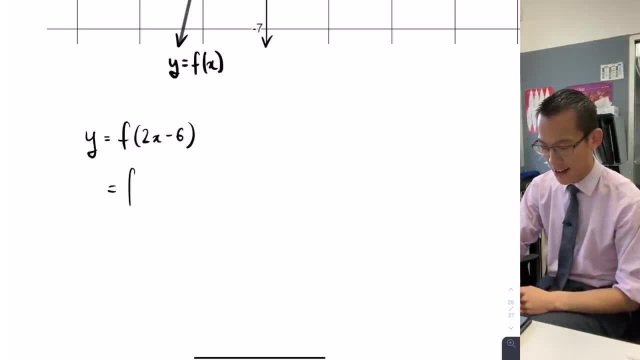 But you're not, which is very sneaky. right Underneath this, on the next line, that minus 6 is not actually acting directly on the x, I want you to imagine kind of like: have you ever seen like a rugby union game right? 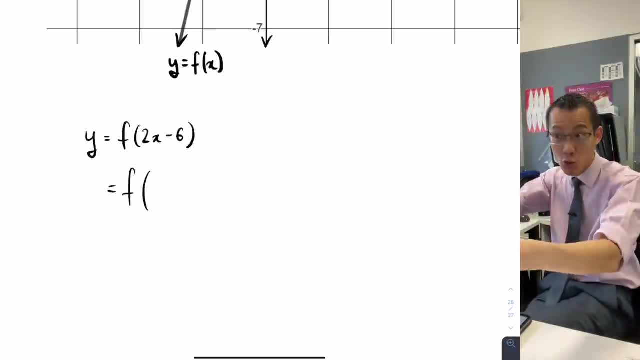 And the ball goes on the ground, and then they all get in this big pile, big scrum right And they're all trying to push the ball back and forth. Okay, Yeah, So you've got people who are really close to where the ball is and they're pushing. 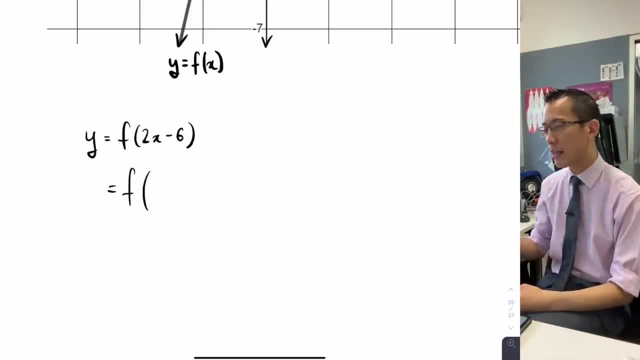 directly on the other team, okay. And then you've got like people all the way at the back and they're pushing as well, but their pushing is kind of indirect right. They're pushing people who are pushing, people who are trying to act on this right. 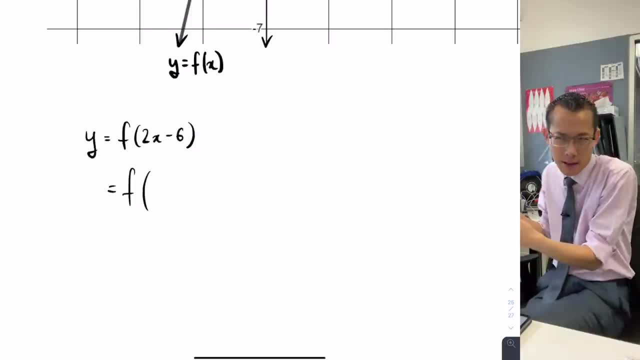 So the further back you are, it's like, oh, like they have less of an impact, as it were. Yeah, That minus 6,, if you like, it's kind of further away from the x. so what we should really write is a factorization here. 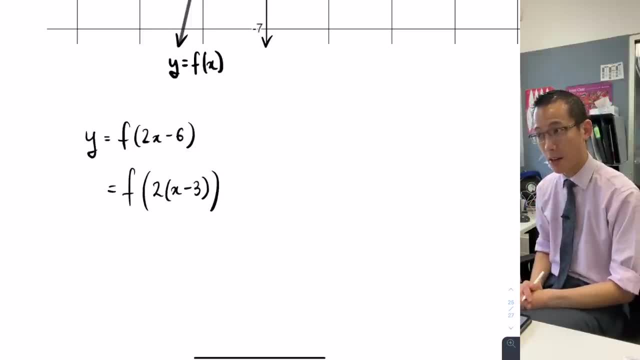 It's really 2 outside of x. It's minus 3.. So can you see now that minus 3 is actually directly acting on x? There's no 2 in the way, okay? So you know how we said: okay, the 2 means it's half the width. 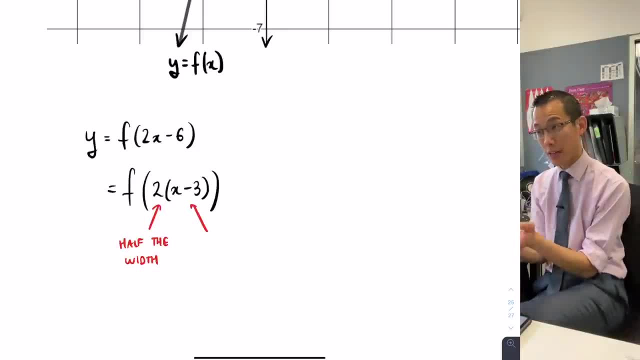 We already wrote that down up above, but now let's put it together. Now we know that the translation is not going to be 6 units, it's going to be 3, okay, We also know it's horizontal because it's changing the x. but I'm going to ask you. 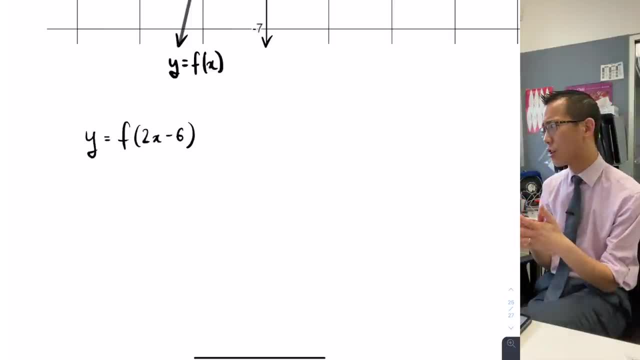 But that minus 6, it sort of seems like, okay, you're going to move 6 units, right, But you're not, which is very sneaky right Underneath this on the next line, that minus 6 is not actually acting directly on the x. 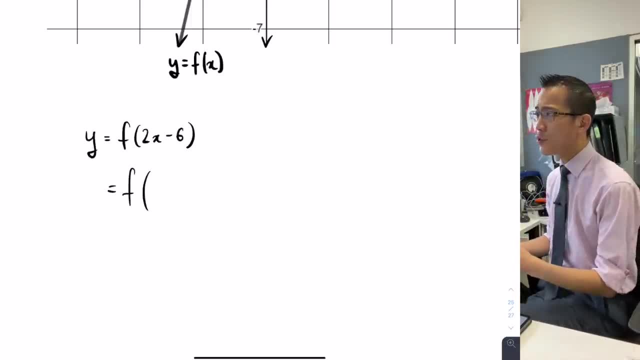 I want you to imagine kind of like – have you ever seen like a rugby union game, right, And the ball goes on the ground and then they all get in this big pile, big scrum, right, And they're all trying to push the ball back and forth. okay, 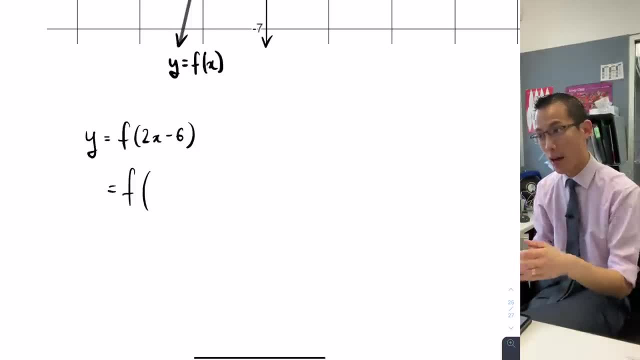 Now there's some people who are really close to where the ball is and they're pushing directly on the other team, okay. And then you've got like people all the way at the back and they're pushing as well, but their pushing is kind of indirect, right. 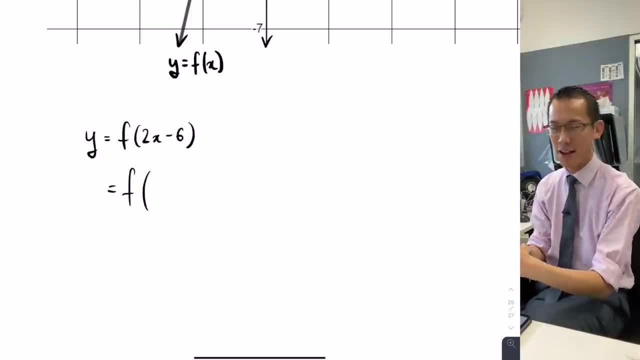 They're pushing people who are pushing people who are trying to act on this right. So the further back you are, it's like, oh, like they have less of an impact, as it were, And that minus 6,, if you like. 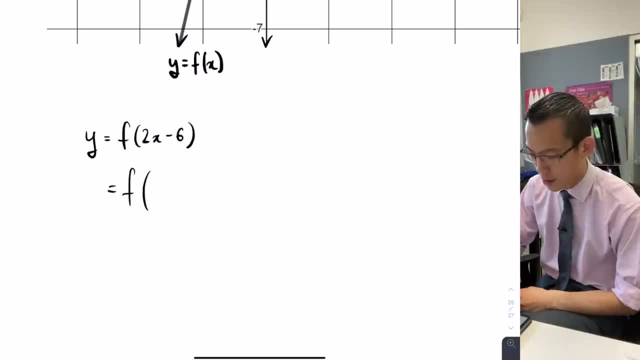 it's kind of further away from the x, so what we should really write is a factorization. here It's really 2 outside of x minus 3.. So can you see now that minus 3 is actually directly acting on x? There's no 2 in the way, okay. 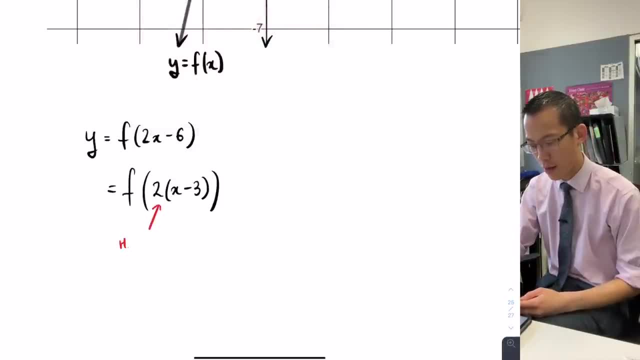 So you know how we said: okay, the 2 means it's half the width. We already wrote that down up above, but now let's put it together. Now we know that the translation is not going to be 6 units, it's going to be 3, okay. 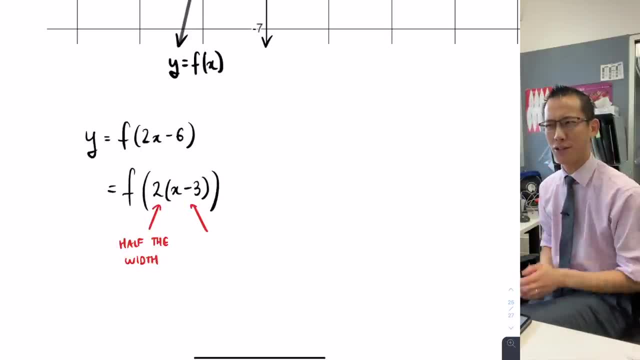 We also know it's horizontal because it's changing the x. but I'm going to ask you: is it left or is it right? What do you think? South, right, And it gets to the right. Okay, It's distinct, right. 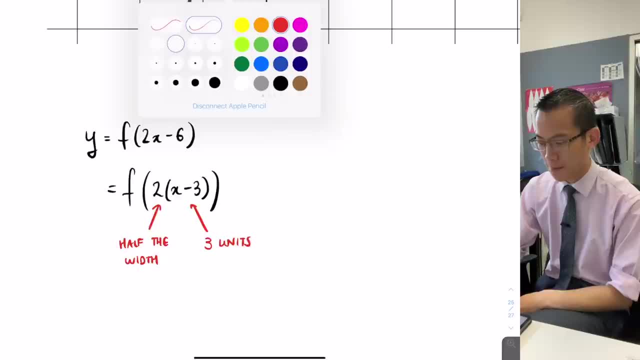 Now the way I remember like which one it is is: if you know, you don't have to write this down, but if you know what this looks like. y equals x squared. do you have a picture in your head of what that parabola looks like? 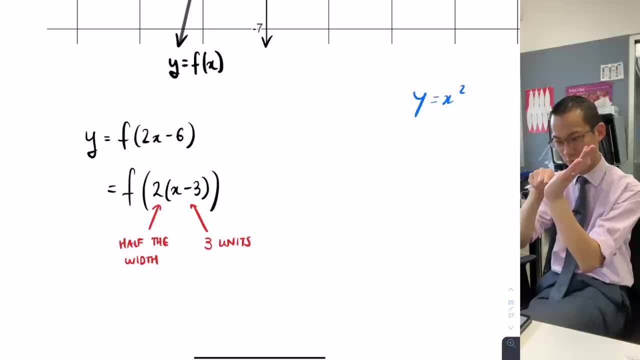 So it's concave up, it's got its little, the vertex, that spot at the bottom, it's at the origin. okay. Now if I compare that to something like let's do this right, What would that look like? okay, 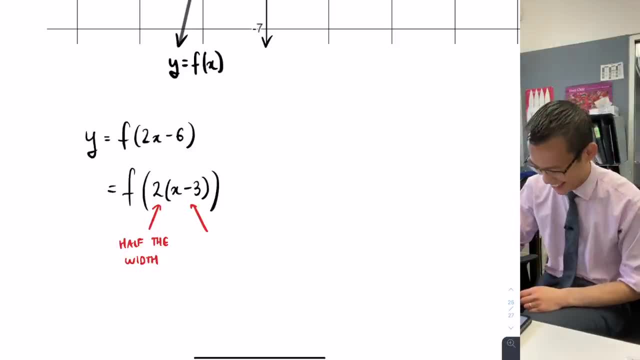 is it left or is it right? What do you think? Ah, Sorry, No, it's right, So it's. I think it's to the right, Like hey, good instinct right Now. the way I remember like which one it is is if you know, you don't have to write. 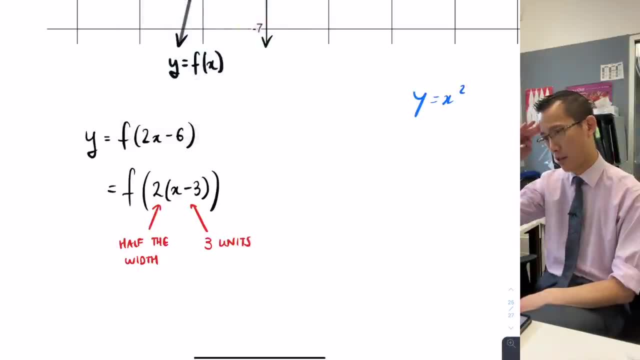 this down. but if you know what this looks like- y equals x squared- do you have a picture in your head of what that parabola looks like? So it's concave up, it's got its little. the vertex, that spot at the bottom, it's at the. 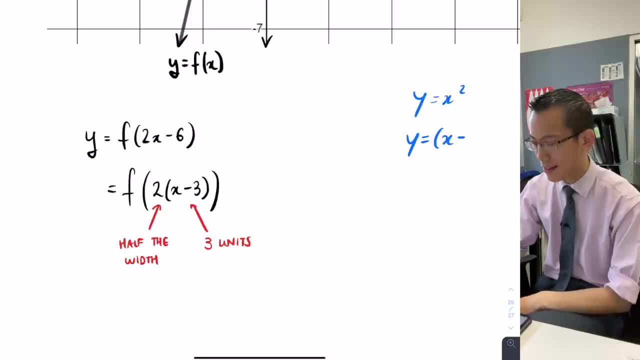 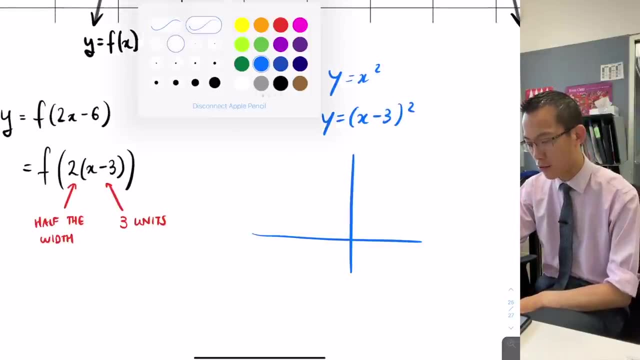 origin. okay, Now, if I compare that to something like: let's do this, right, What would that look like? okay, Now, I am going to draw it for you, You don't have to. The original graph looks like this: 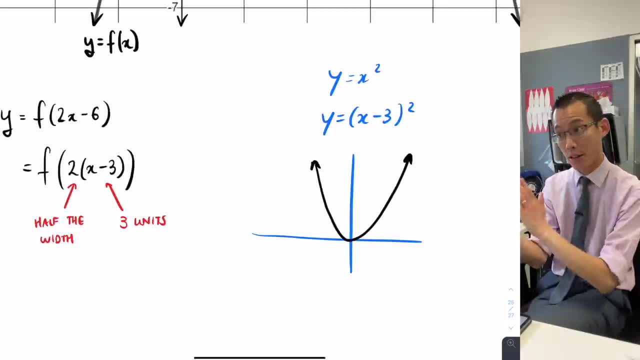 X minus three all squared. it's different because there's a horizontal translation. Where's the new intercept? Like it's not going to be here at zero zero, Where's it going to be? I have a think I need to think about. what value of x- sorry, it's on the wrong spot- what value of x do? 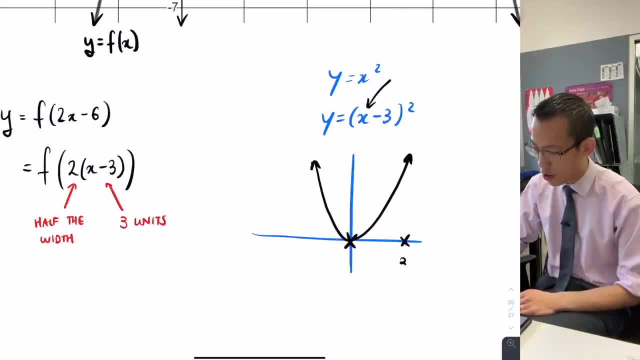 I put in: Ah, Positive three, Yeah, it's a positive three, right? So I would go: oh, it's over there, and then I draw the rest of the shape. It's actually going to be less than three. 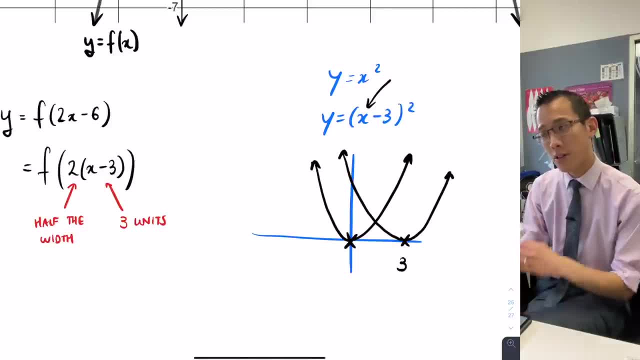 So ideally I would draw myself out here. it's going to be less than three into half Now. you would notice that this saying has moved me a bit to the right. I'm just gonna go with this here: Positive three. that has moved to the right, exactly like what you said, this guy will as 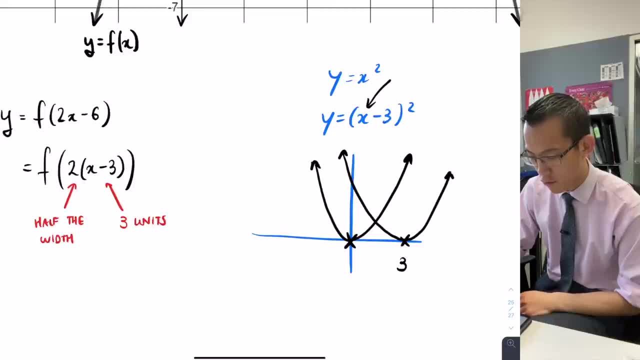 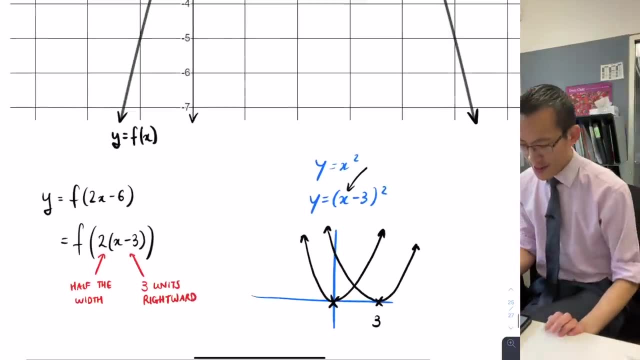 well. So everything is kind of backwards. You're like: oh this multiplying by two doesn't make you twice as big, it makes you half. And this minus three doesn't move you to the left, moves you to the right. So everything is kind of weird and reversed. 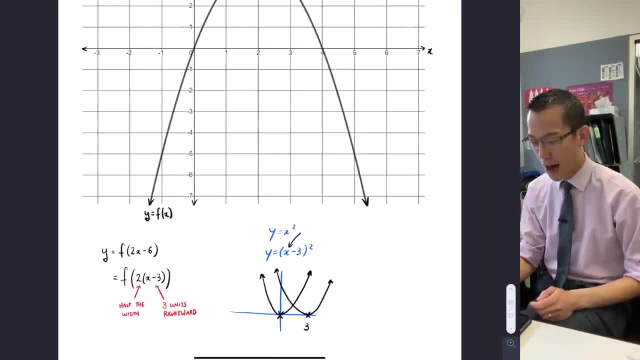 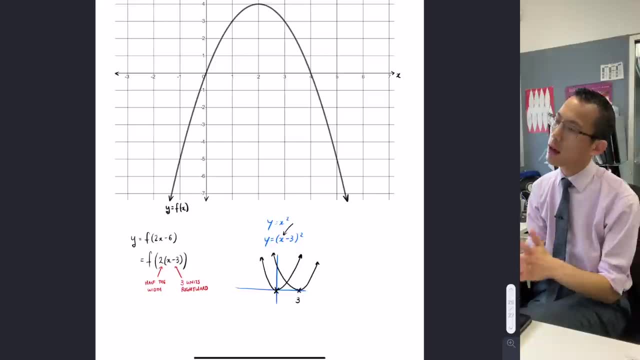 So three units Rightward, I guess, is the way I'd say it. Okay, we've got this graph. I know the two things we need to do. We've got to do a dilation, We've got to do a translation. Okay, there's one last question, which is: which one do you do first? 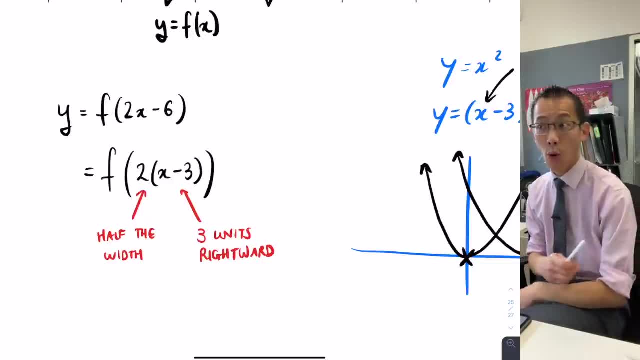 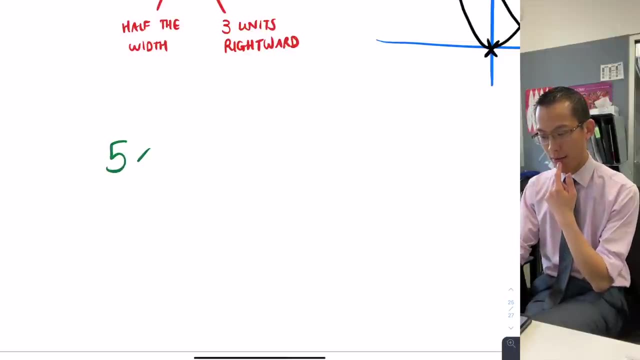 Okay, because If you think about your order of operations, If you do operations in different order, you get different answers, right? Yeah, exactly Like if let's just um think about a numerical example here, right? If I said to you: Can you please tell me what is five times three? take away one. 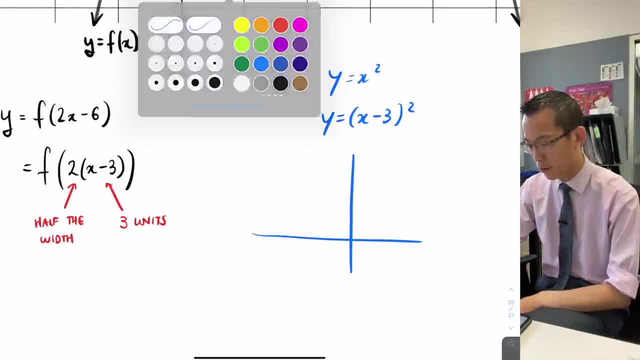 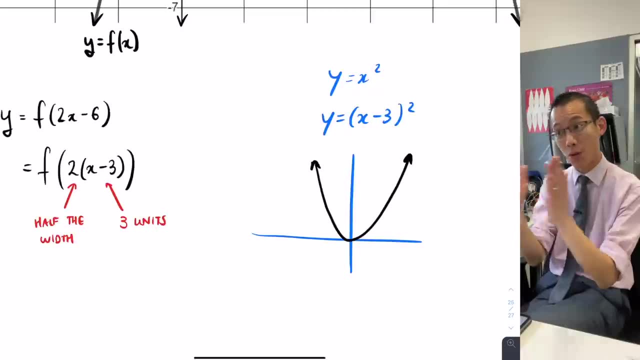 Now I am going to draw it for you. you don't have to, but the original graph looks like this: x minus 3 all squared. it's different because there's a horizontal translation. Where's the new intercept? Like it's not going to be here at 0, 0.. 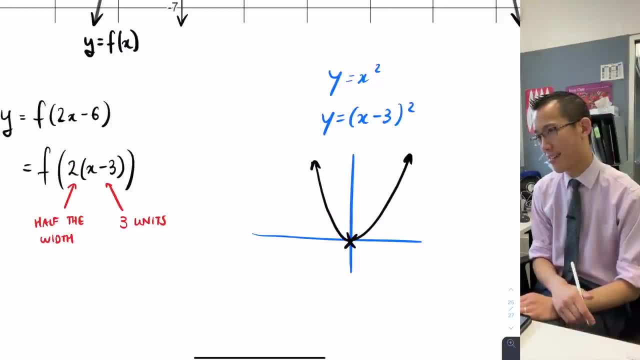 Where's it going to be? I have a think I need to think about. what value of x- sorry, it's on the wrong spot- What value of x do I put in Positive 3.. Yeah, it's a positive 3, right. 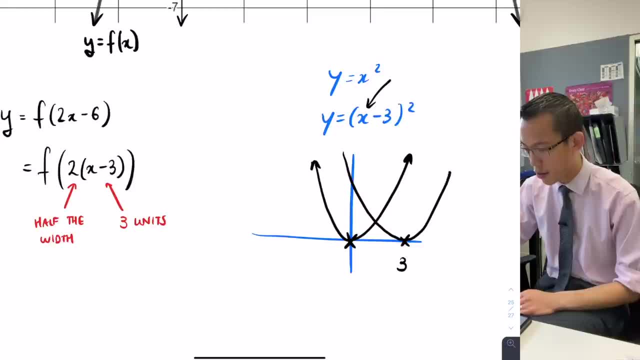 So I would go: oh, it's over there, and then I draw the rest of the shape So you can clearly see that has moved to the right, exactly like what you said. this guy will as well. So everything is kind of backwards. 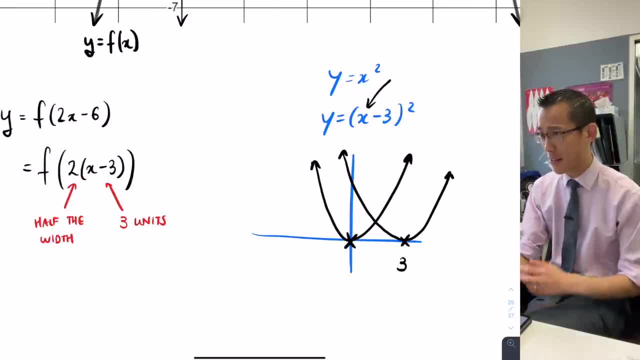 You're like: oh, this multiplying by 2 doesn't make you twice as big, it makes you half. And this minus 3 doesn't move you to the left, it moves you to the right. So everything is kind of weird and reversed. 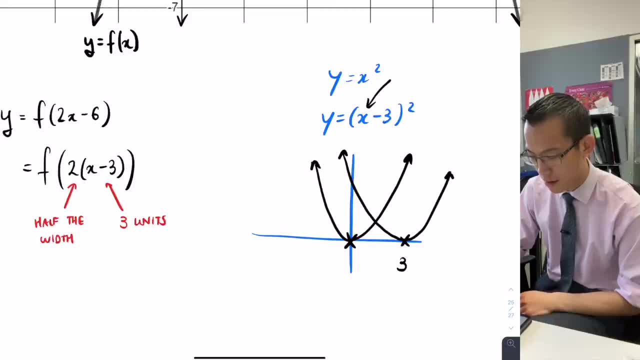 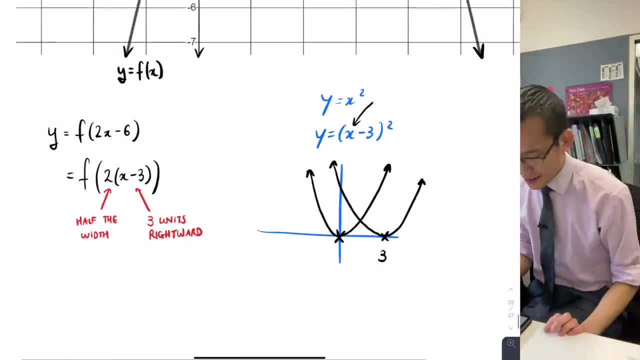 So 3 units rightward, I guess, is the way I'd say it. Well, upward, downward, leftward, rightward, okay, Right, so we're going to do these two changes. okay, We've got this graph. 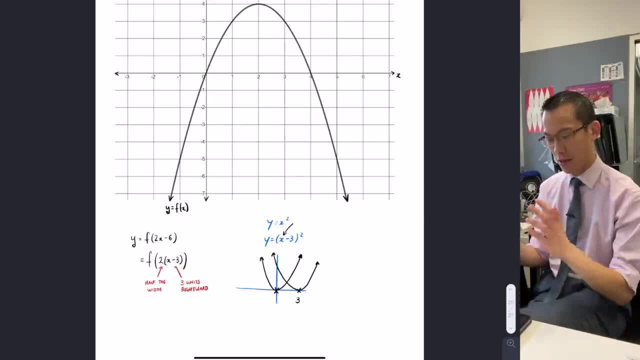 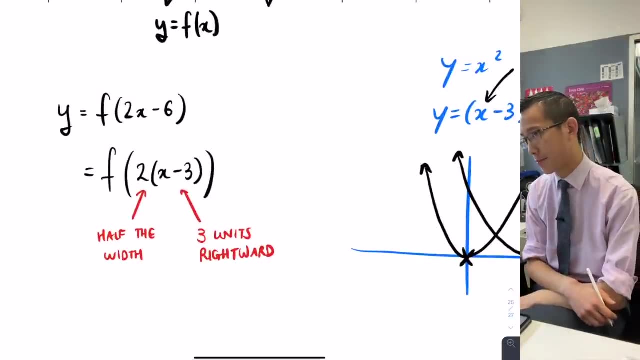 I know the two things we need to do. We've got to do a dilation, we've got to do a translation. okay, There's one last question, which is: which one do you do first? Because if you think about your order of operations, 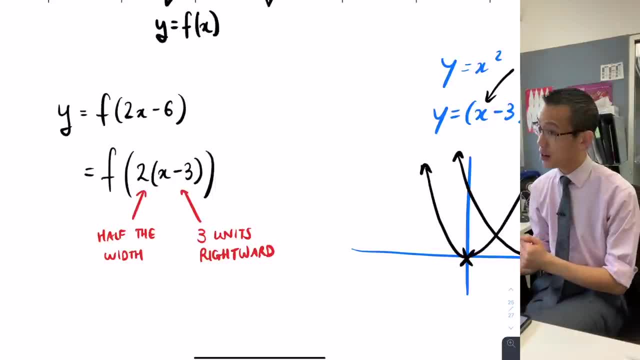 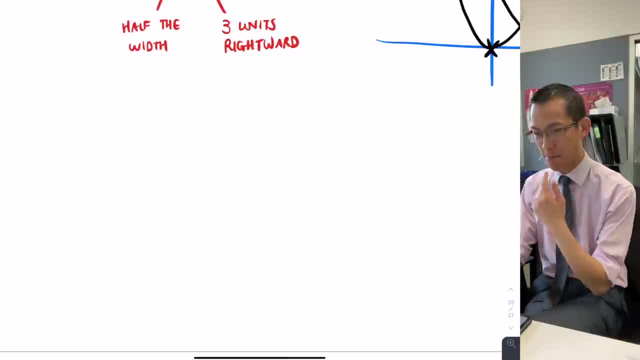 if you do operations in different order, you get different answers, right? Yeah, exactly, Let's just think about a numerical example here, right? If I said to you, can you please tell me what is 5 times 3, take away 1, right? 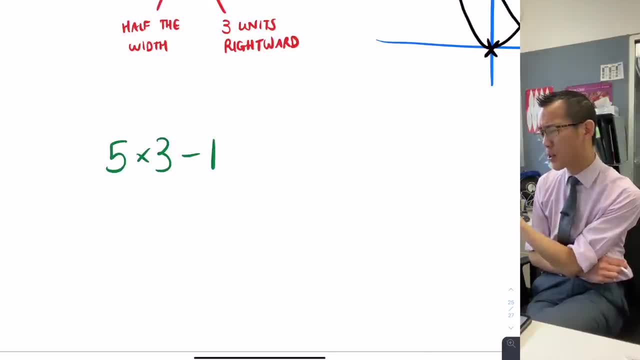 You've got two operations there, yeah, Yeah, And depending on which one you do first, you get a completely different answer, right? We know what the order of operations are. We're like: oh, you multiply first, right, And then you do your subtraction, okay? 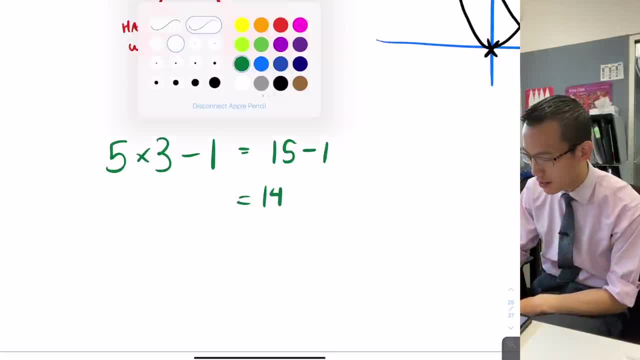 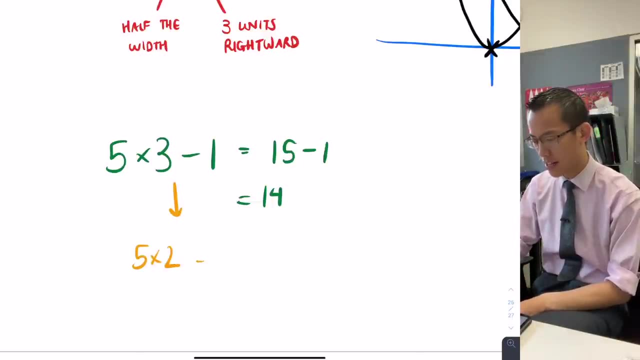 I hope you can see here, though, if I did it in the wrong order, it just completely goes. yeah, it's very confusing, right? You're like: oh, if I do my subtraction first, I get 5 times 2, and that's 10.. 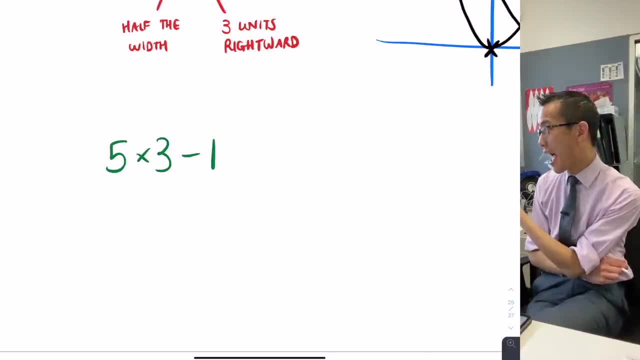 Right, you got two operations there, Yeah, and Depending on which one you do first, you get a completely different answer, right? We know what the order of operations are. We're like: oh, you multiply first, Right, and then you do your subtraction. Okay, I hope you can see here, though, if I did it in the wrong order. 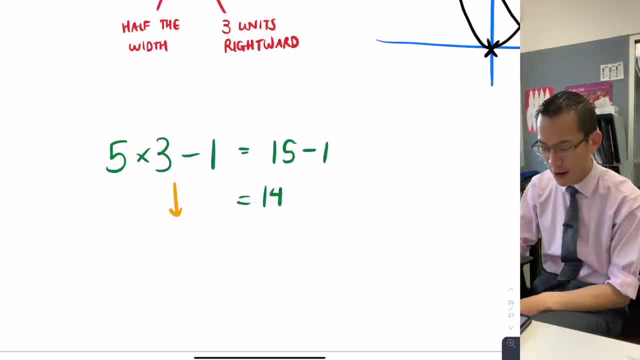 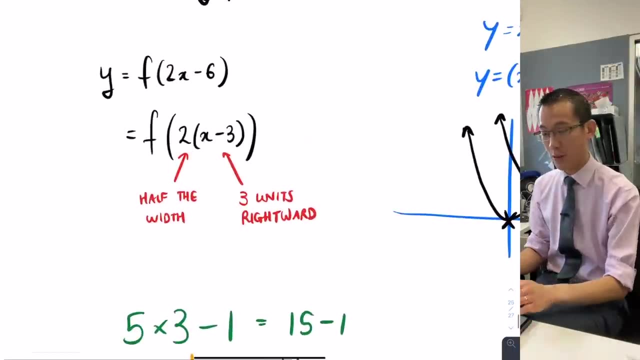 It just completely goes. Yeah, it's very confusing right? You're like: oh, if I do my subtraction first, get five times two, And that's ten. you're like: what, which one is it? Okay, so we have to work out which one is first. 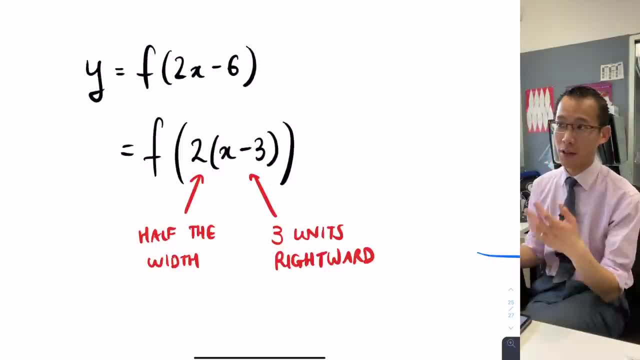 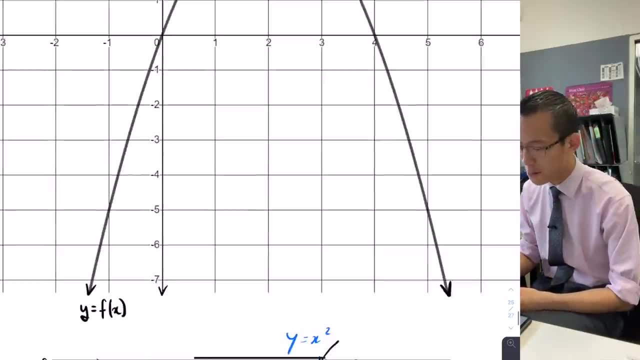 Yeah, thankfully for us, the order of operations with numbers is exactly the same as the order operations with graphs. So which one which we do first? we do half the width first, Okay, so let's go. Let's have a look now. This is the graph, and 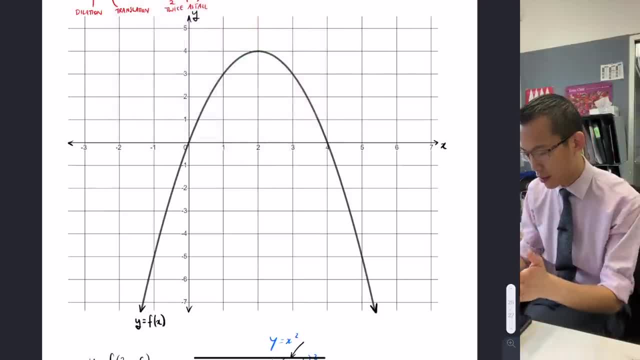 What we do. the easiest way to do this is- and whichever color you want is fine When they provide it to you. If they don't give you an equation like tell you: this is y equals x squared, whatever they have to give you, give you grid lines, like I've presented to you, because you've got to work out. 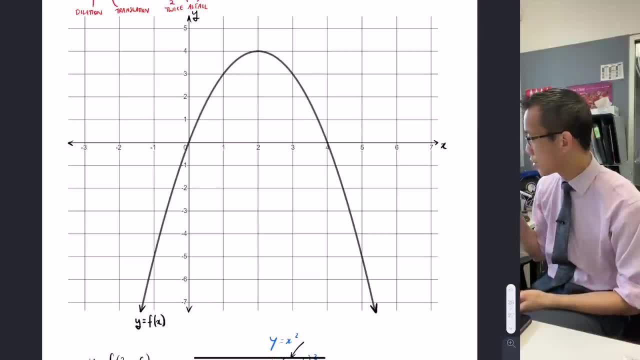 points on the graph and then use those points to help you. So I want you to look and tell me which parts of the graph can you see lie on like some nice, neat coordinates. Can you see any that are easy to point out? Well, you can, you could. 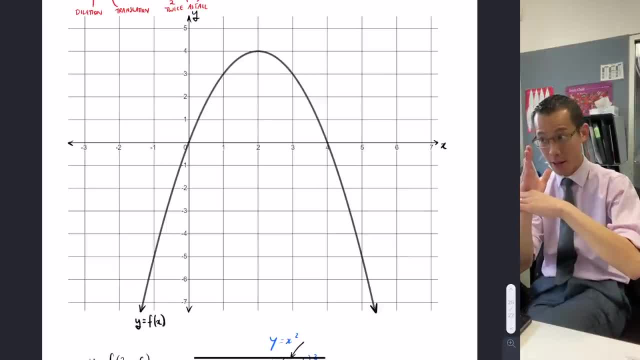 give me a stationary point, if you like. I'm really looking for things that line up on grid lines, because then I know what numbers they are and then I can do this halving and translating all the rest. So pick any point you like. Yeah, fantastic, So I've got two intercepts. very good, So the intercepts. 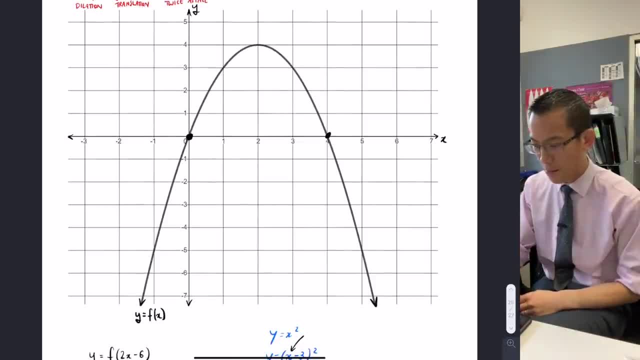 are at zero and four, So let's just start with those zero and four, okay, And we will definitely. you're using blue, so I'll use blue as well, okay. So silly, silly question to ask, but it's not rhetorical. I'm halving the width of this, right, So 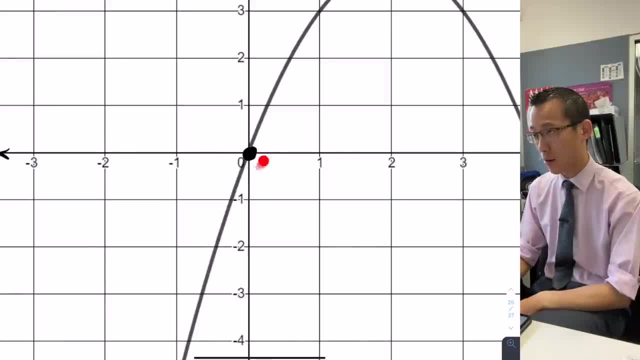 the X value for this first intercept here is zero. What's half of zero? Still zero. So I'm going to put an X right there. okay, That point is when I, when I dilate it, it doesn't go anywhere. yeah, Now when it goes to the 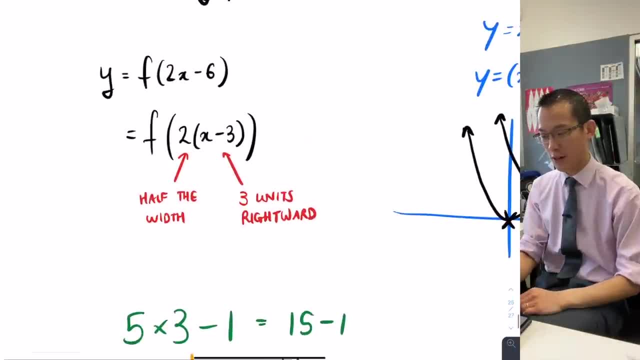 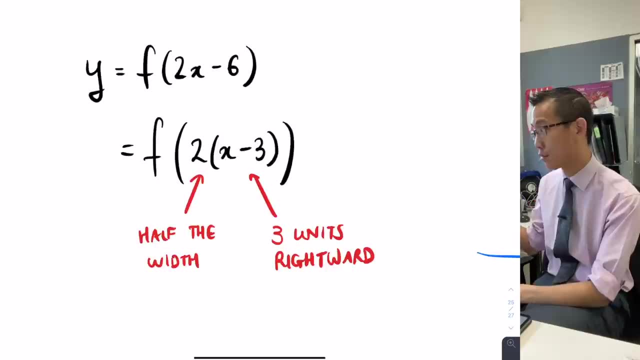 You're like: what, Which one is it? okay, So we have to work out which one is first. Yeah, Thankfully for us, the order of operations with numbers is exactly the same as the order of operations with graphs. Okay, So which one should we do first? 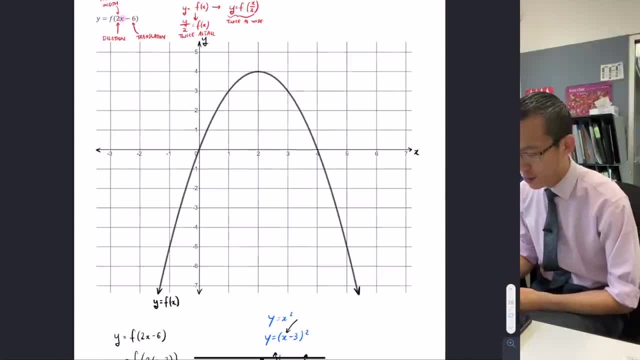 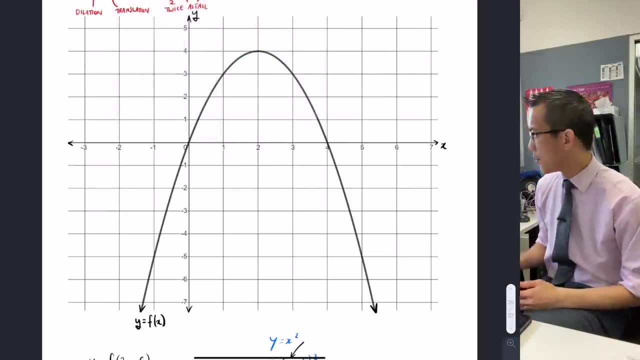 We need to do half the width. We do half the width first. Okay, so let's go. Let's have a look Now. this is the graph And what we do. the easiest way to do this is: and whichever color you want is fine. 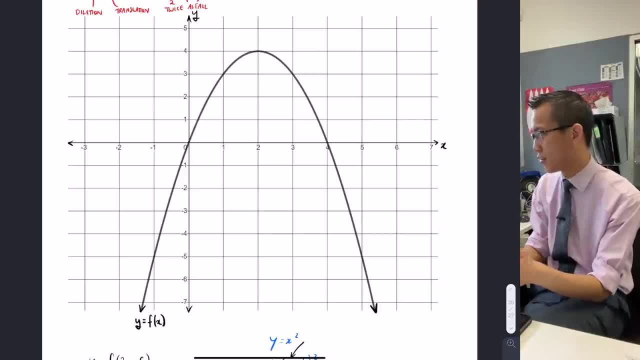 when they provide it to you. if they don't give you an equation like tell you this is y equals x squared, whatever, they have to give you grid lines, like I have presented to you because you've got to work out. 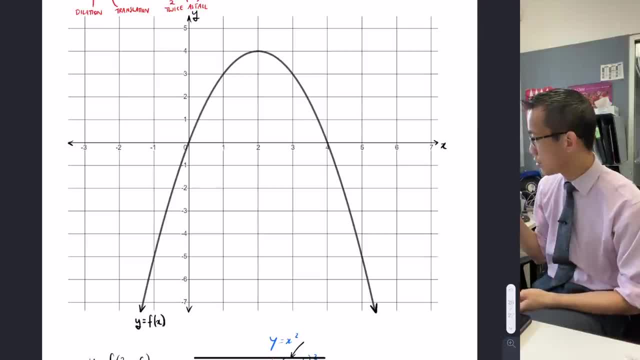 what are the points on the graph and then use those points to help you. So I want you to look and tell me which parts of the graph can you see lie on like some nice, neat coordinates? Can you see any that are easy to point out? 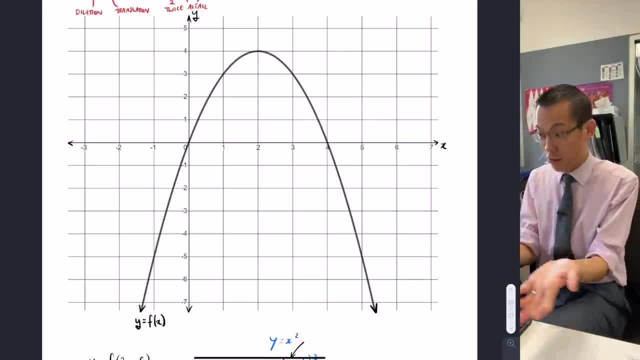 As in like stationary points. Well, you could give me a stationary point if you like. I'm really looking for things that line up on grid lines, because then I know what numbers they are and then I can do this halving and translating and all the rest. 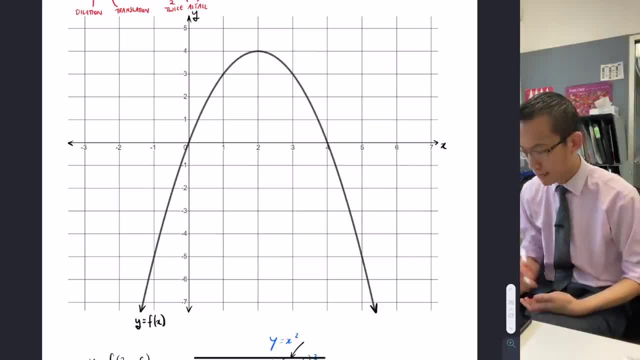 So pick any point you like. Well, it kind of intersects the x-axis- Yeah, fantastic. So I've got two intercepts. Four, That's very good. So the intercepts are at zero and four. So let's just start with those. 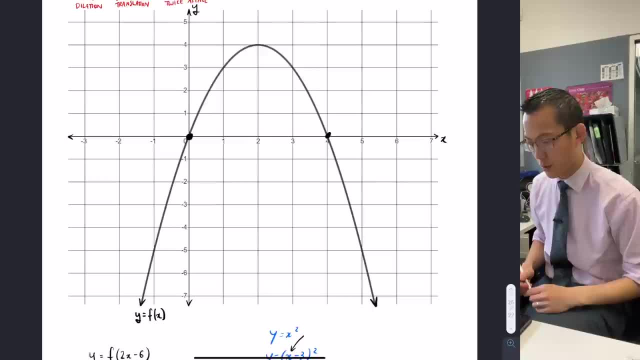 Zero and four? Okay, And we will definitely. you're using blue, so I'll use blue as well, Okay. So silly question to ask, but it's not rhetorical. I'm halving the width of this, right, Yeah? 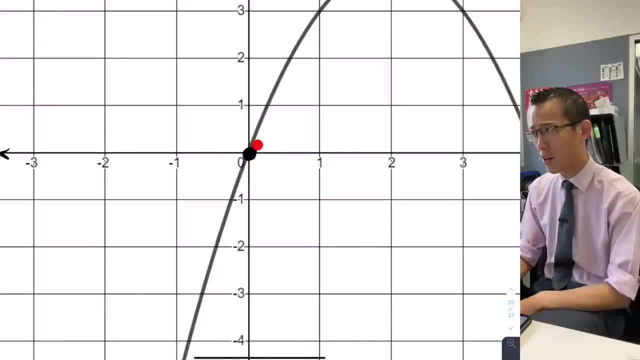 So the x value for this first intercept here is zero. What's half of zero? Still zero, Still zero. So I'm going to put an x right there. Okay, That point. when I dilate it, it doesn't go anywhere. 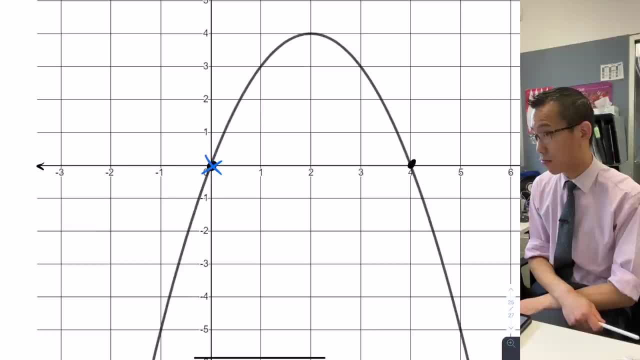 Yeah, Now, when it goes to the other intercept, you're like: oh, it's four, So I'm halving everything, right? So what is it now? It'll be intercepting at two. It'll be intercepting at two. 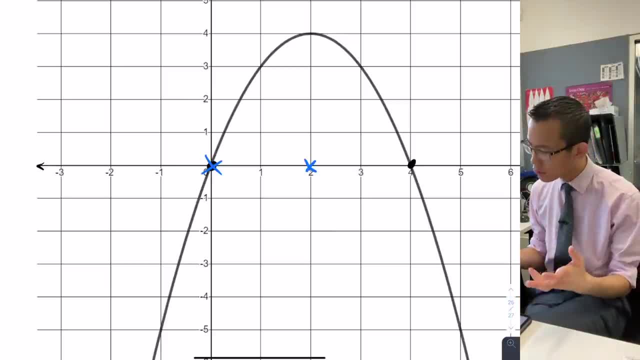 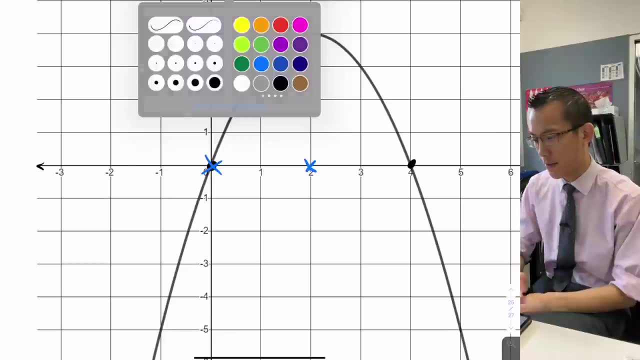 Very good, Okay, So I'll put an x there. Find me some other points. What's another point on the graph? Like you've got your intercepts Great. Are there any other points that you can see line up nicely, Like the top of the curve? 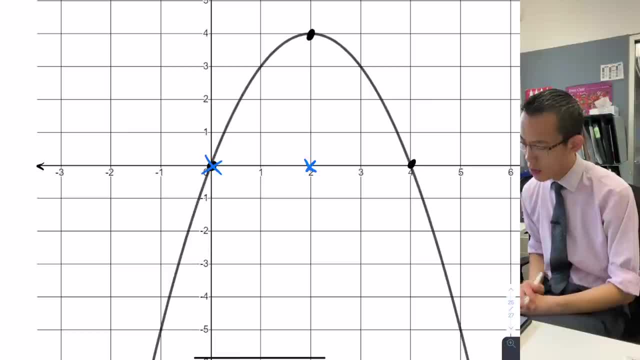 Yeah, The top of the curve, the vertex right, So we would say its x coordinate is two. So I'm going to halve that and I'm going to make it one Very good, And you can sort of continue this process right. 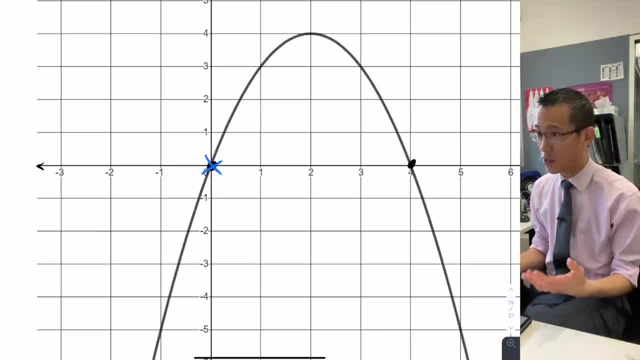 other intercept. you're like: oh, it's four, So I'm halving everything, right. So what is it now? It'll be intercepting at two. Very good, okay. So I'll put an X there. Find me some other points. What's another point on the graph? Like you've got your. 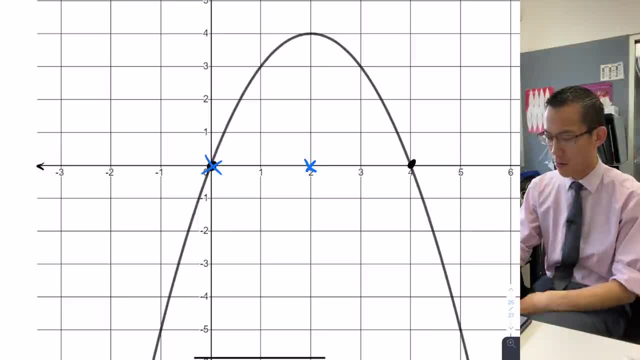 intercepts, great. Are there any other points that you can see line up nicely, Like the top of the curve? Yep, the top of the curve, the vertex right. So we would say its X coordinate is two. So I'm going to halve that. 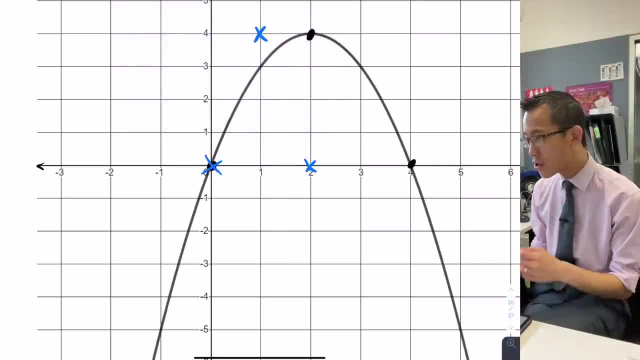 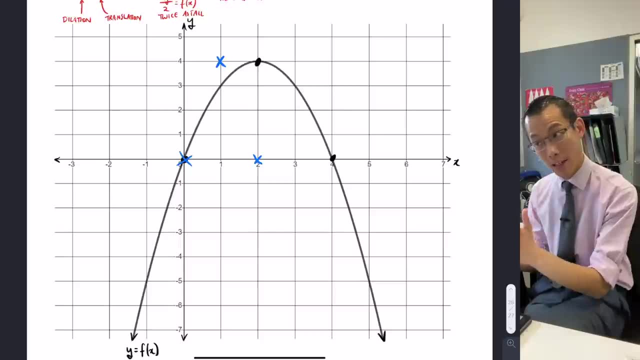 And I'm going to make it one Very good, And you can sort of continue this process, right, I'm gonna pause for a minute and let you find as many nicely aligned spots and then see where they actually should go to when you halve them, okay. 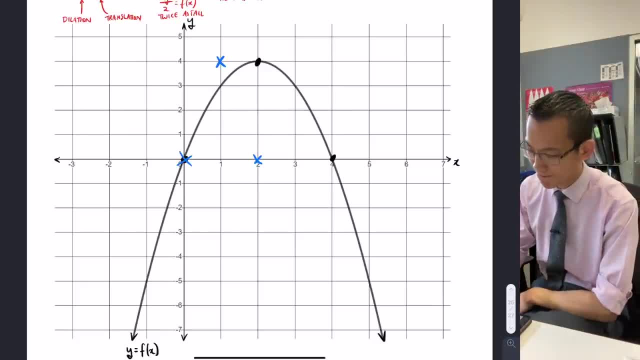 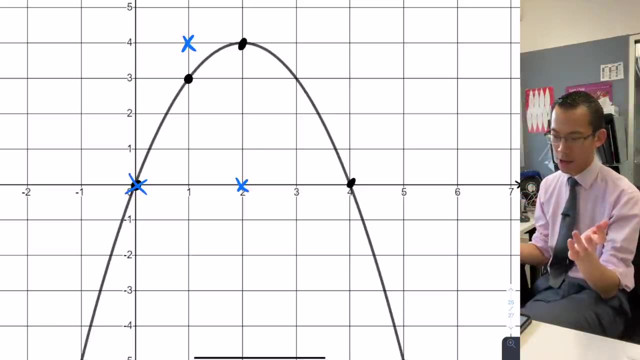 Have a think. What other ones do you see? There's one quite close to that vertex. you can see there, right, Quite close to the top, a couple actually, Yeah. so you've got this x value here is 1. and then you've also got um. parabolas are symmetrical, yeah. so if you've got 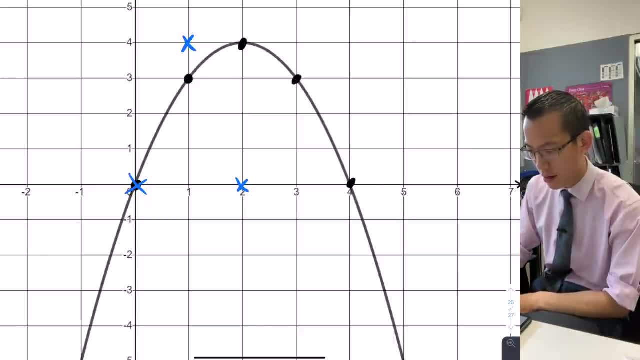 one on the left, yeah, you can see it on the other side. so what x value is that one on the right hand side? three, that's three, very good, so we want to halve both of those. so the first one is one. it's going to halve, to be half, very good. a half of one is half good, um, and then a half of three. 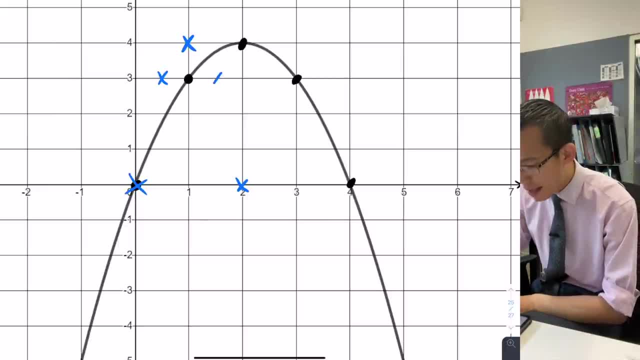 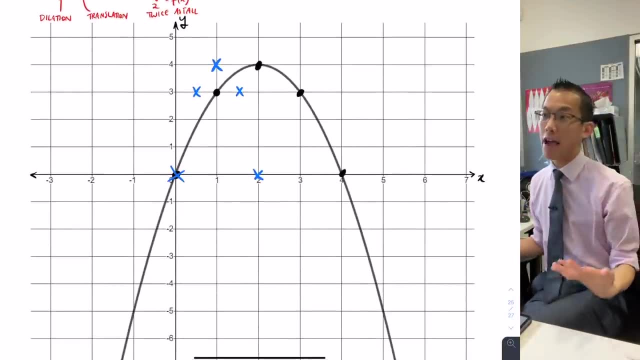 one and a half cool. and now, just before we go any further, um, because we're sort of getting to the point where we've got a good picture here, um, you can see. you're like: oh, the parabola i had before you're starting. can you see where the blue dots are going to line up? you're like: oh, i have another. 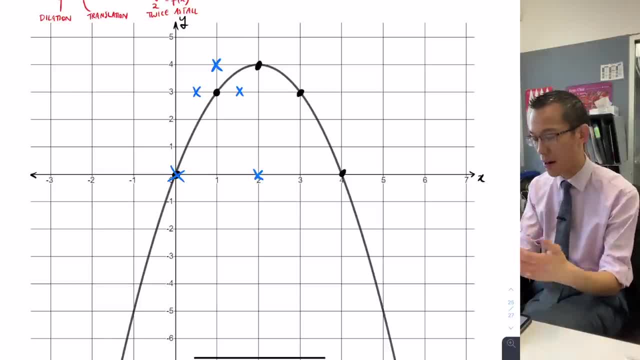 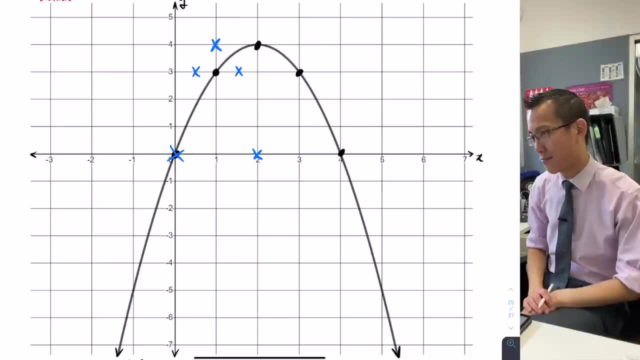 parabola, but it's just skinnier, which is kind of what i wanted. right, i want to halve the width. um, i gave you quite a lot of vertical um scale here. can you see one other spot which also has this mirror? yeah, very good. so what's that x value over there? uh, negative one. yeah, negative one. so 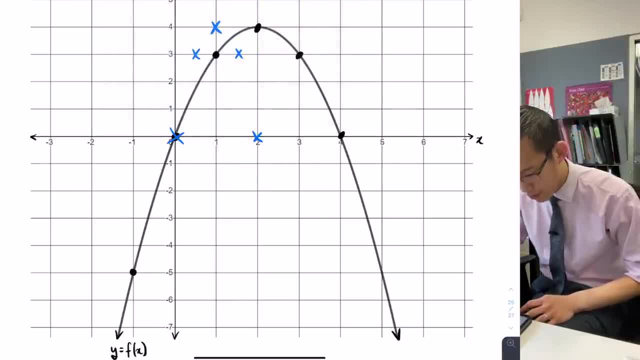 what's half the width? negative, half negative, half, very good. and then there's, yeah, there's, the symmetrical version. so that's it: x equals what? five? five. so you halve it and you get x equals two and a half. very good, okay. so, um, it looks to me at least. when i designed this, i was: 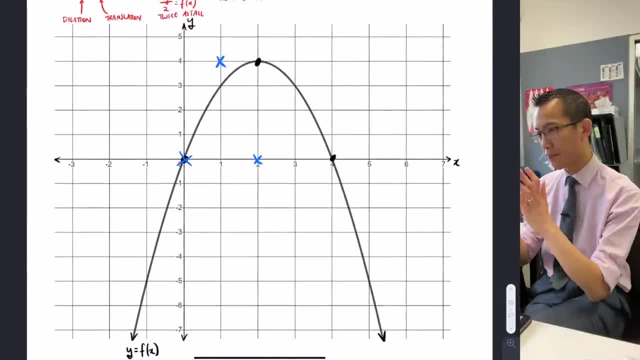 I'm going to pause for a minute and let you find as many nicely aligned spots and then see where they actually should go to when you halve them. okay, Have a think. What other ones do you see? There's one quite close to that vertex. 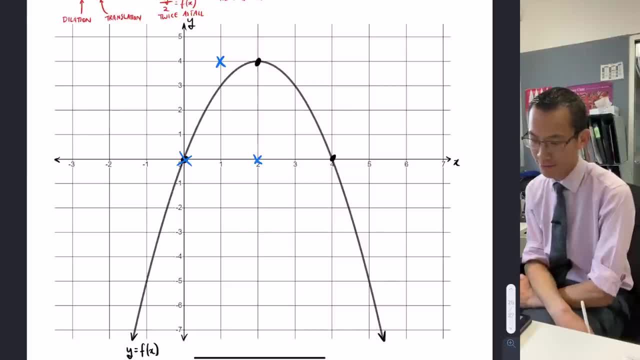 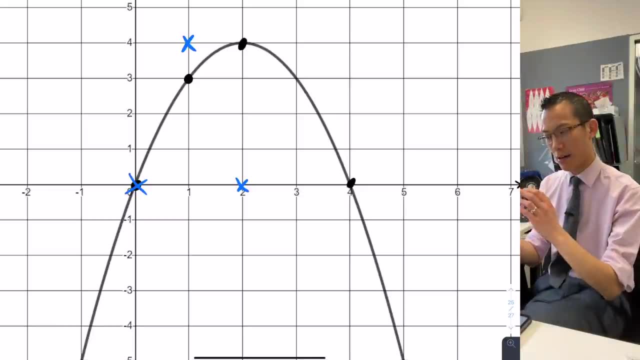 You can see that right, Quite close to the top. A couple, actually These ones, Yeah. So you've got this x value. here is one, Yeah, And then you've also got this x value. here is one. Parabolas are symmetrical, yeah. 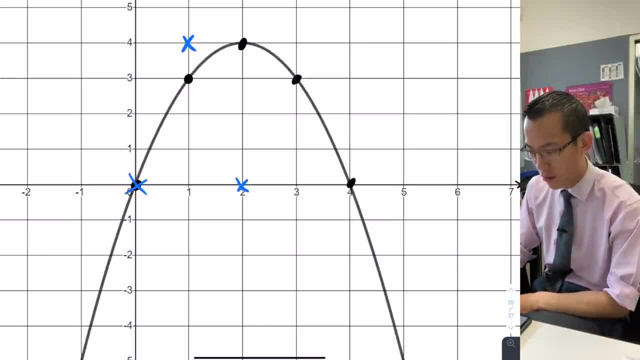 So if you've got one on the left, yeah, you can see it on the other side. So what x value is that one on the right-hand side? Three, That's three. Very good, So we want to halve both of those. 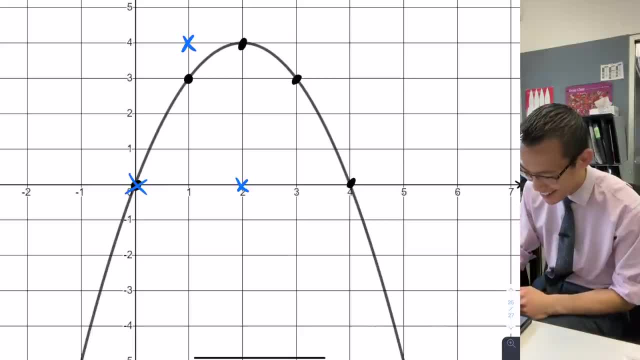 So the first one is one. It's going to halve, to be Half, Half, Very good. A half of one is half Good, And then a half of three, One and a half, One and a half Cool. 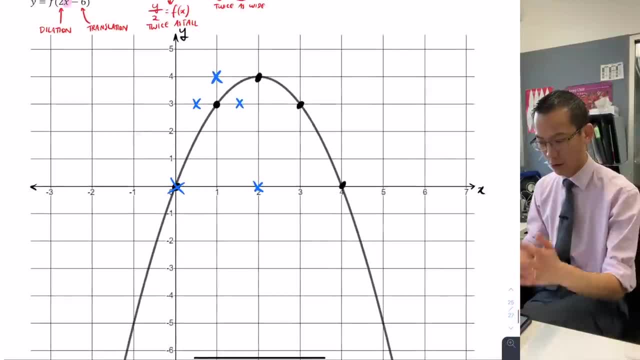 And now, just before we go any further, because we're sort of getting to the point where we've got a good picture here, you can see, you're like: oh, the parabola I had before, can you see where the blue dots? 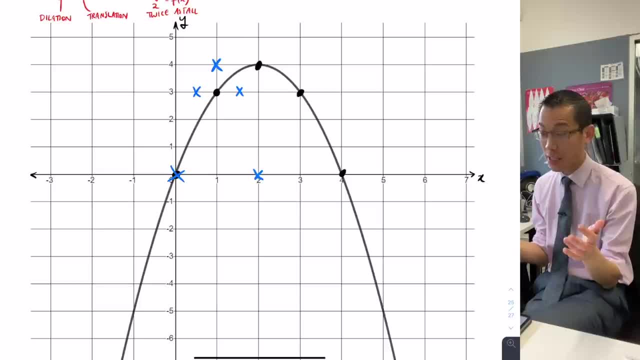 are going to line up. You're like: oh, I have another parabola, but it's just skinnier, which is kind of what I wanted. right, I want to halve the width. I gave you quite a lot of vertical scale here. 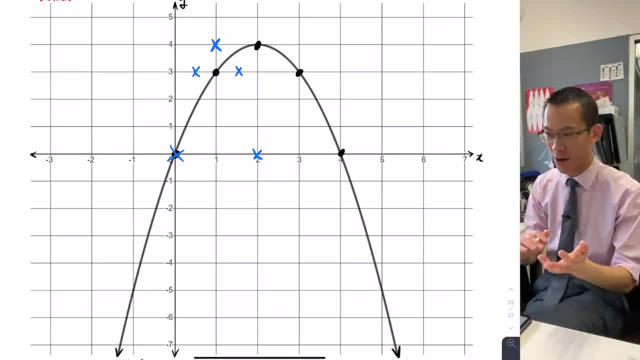 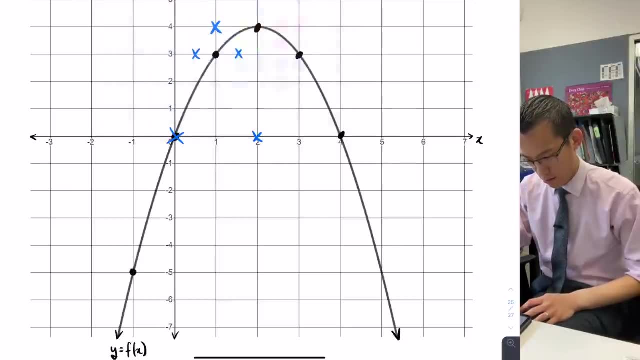 Can you see one other spot which also has this mirror? Yeah, very good. So what's that x value over there? Negative one, Yeah, negative one. So what's half the width, Negative, half, Negative, half, Very good. And then there's yeah. 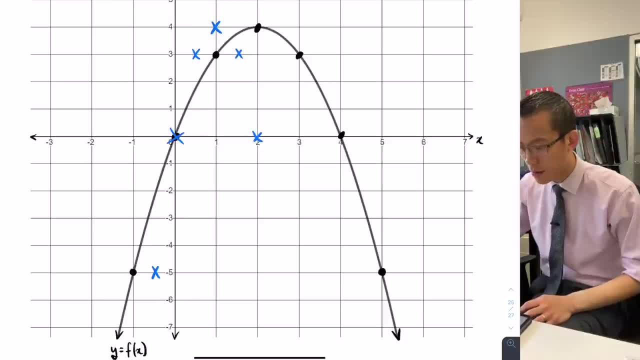 there's the symmetrical version. So that's: x equals what? Five? Five? So you halve it, you get x equals Two and a half. Very good, Okay, So it looks to me at least when I designed this. 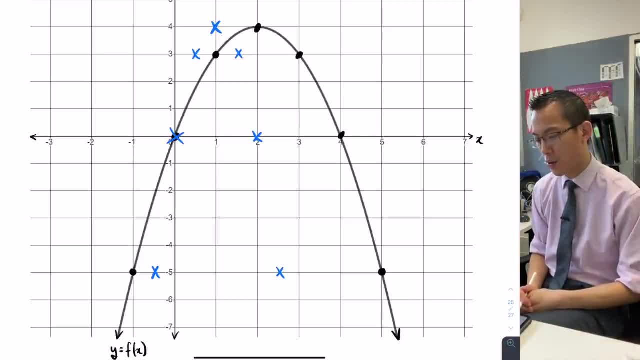 I was like I think that's all of the points that sit nicely, Okay. So what I'm going to do is I'm going to think about: okay, what does this thing look like? I'm not. this is not the actual graph. 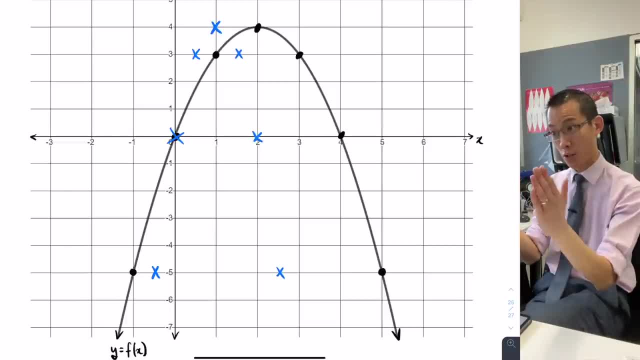 that I'm going to end up with, because I've only done one of the transformations. I've only done the squashing pit. Yeah, I need to do the second one. Yeah, But let's just quickly get a sense for ourselves. I'm just going to draw. 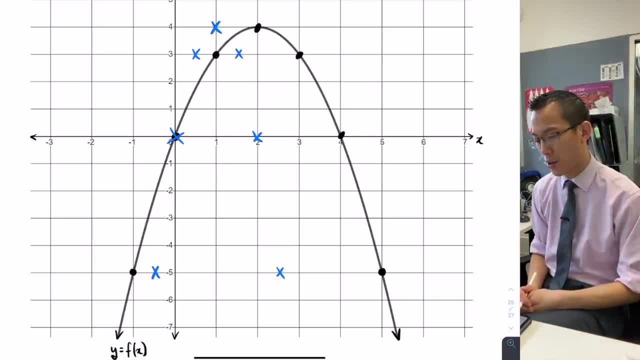 like. i think that's all of the points that sit nicely, okay. so what i'm going to do is i'm going to think about: okay, what does this thing look like? i'm not. this is not the actual graph that i'm going to end up with, because i've only done one of the transformations, i've only done the squashing fit. 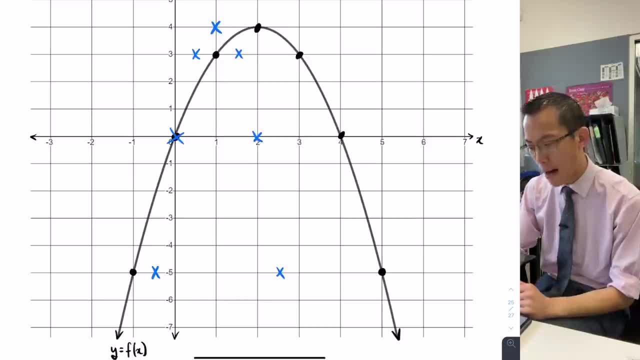 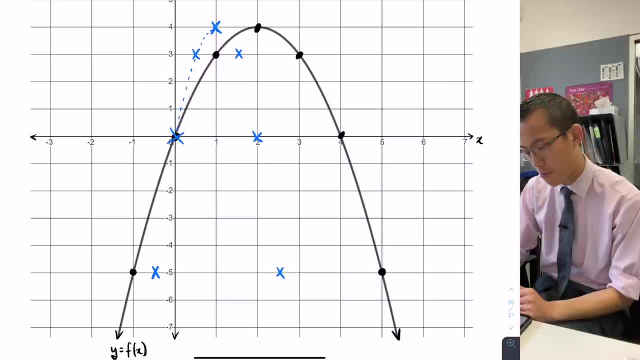 going to draw some dotted lines here. i'm like, oh, if i join the knots, if i connect these right, here is this sort of skinnier looking parabola that we were um hoping to get. so you're like, okay, good, i've done um one of my translations and i guess it sort of keeps on going downwards, like. 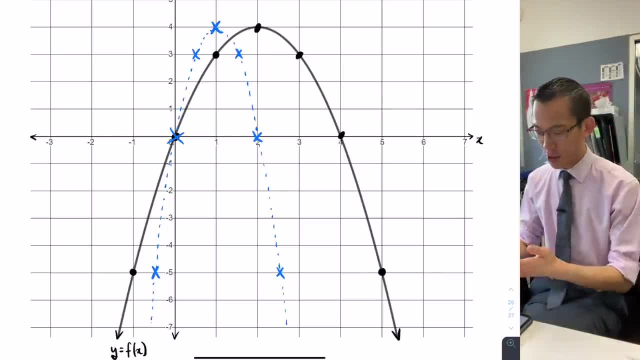 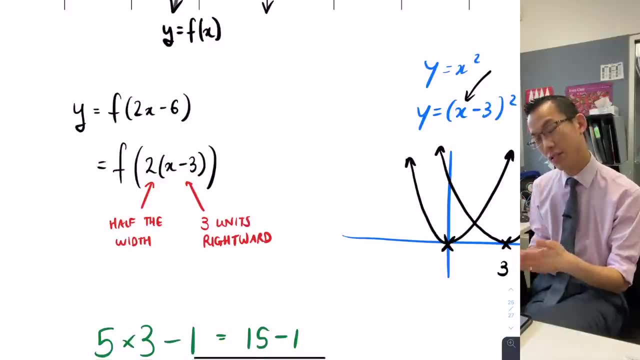 that, okay, okay, fantastic, um, so we've used blue. why don't we switch over to red? okay, we have done the- uh, check it out. we've done half the width, okay, and now we've got to do the other transformation, which is three units to the right, which, in some ways, is even easier than what we did. 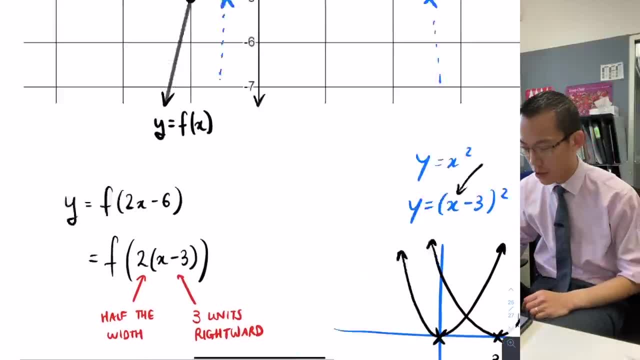 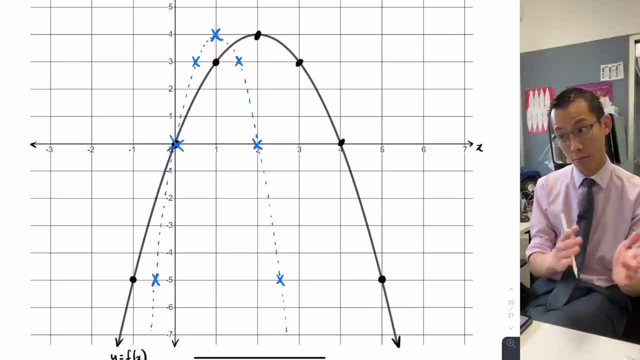 just now because, like, oh, just everything, yeah, just move it right. so, um, it makes sense to take those same. what are we, how many do we get? we had five points, yeah, five points, and to move all of them, three units, okay, um, so let's just go from left to right. um, that first one you can see there on the 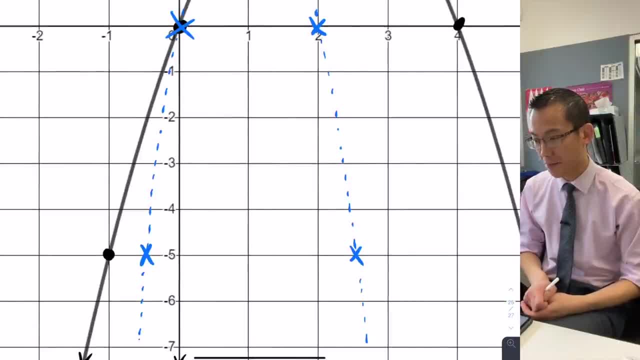 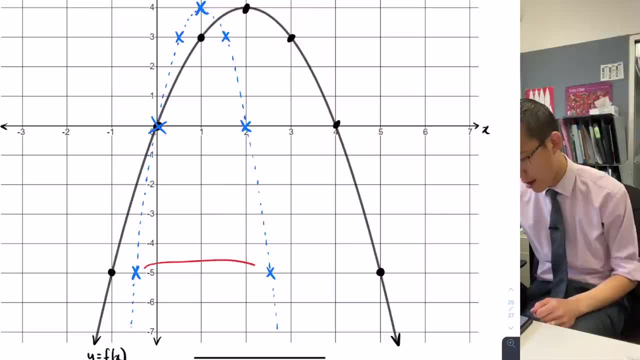 left it's at negative a half, yeah. so when you add three to like where that one is, yeah, it moves to two and a half. that's interesting. so i'm actually going to you don't have to go to the left, you're going to have to put this on yours, but i'm going to show in this other color. i'm moving that guy. 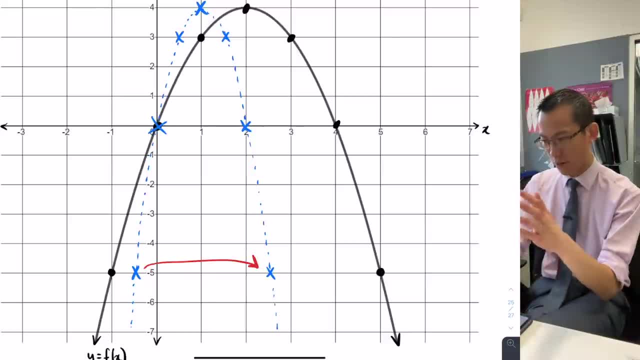 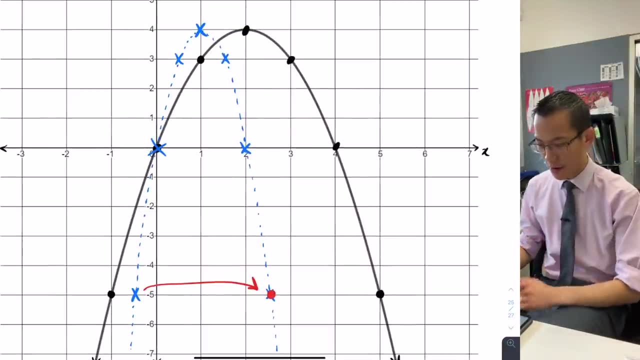 to the right. okay, um, instead of using an x- because i don't want to confuse the stuff here- um, i guess i'll put a big fat dot in in red. okay, all right, um, let's keep on going from left to right. so i've got that. um, that thing at the origin right, so it moves. also three units, everything goes through. 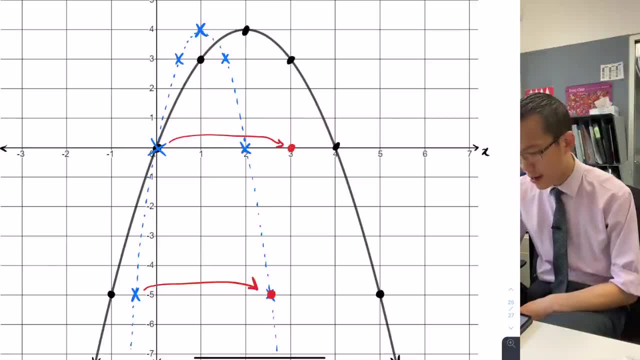 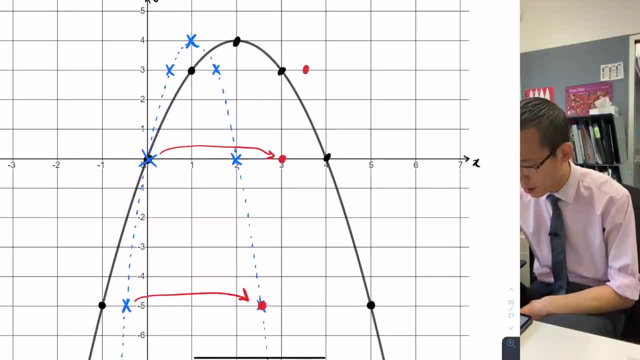 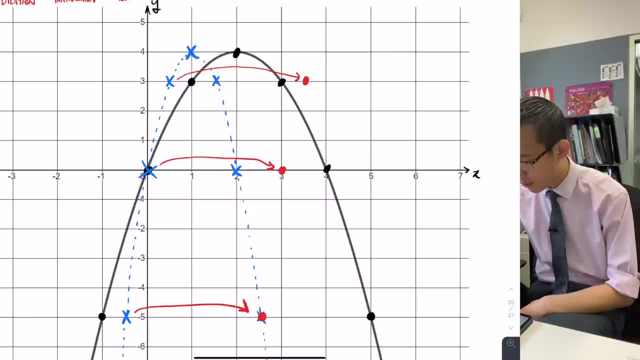 this. so, yeah, it's going to be moved over to three. you're going to keep going, right? you tell me what to do next? um, you move the half to three and a half. fantastic, so there we go. it moves over. you move the stationary point to four. yep, it was at one and now it's at. 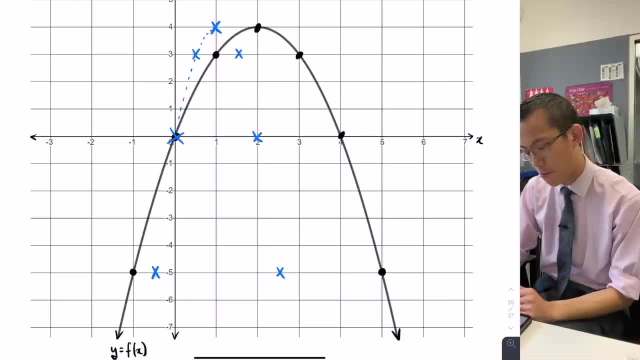 some dotted lines here. I'm like, oh, if I join the knots, if I connect these right, here is this sort of skinnier looking parabola that we were hoping to get. So you're like, okay, good. 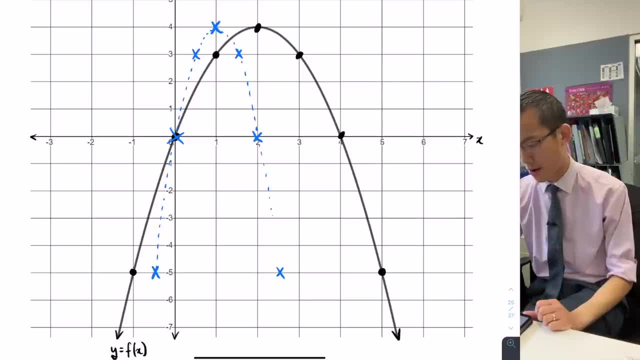 I've done one of my translations and I guess it sort of keeps on going downwards like that. Okay, Mm-hmm, Okay, fantastic. So we've used blue. Why don't we switch over to red? Okay, We have done the. 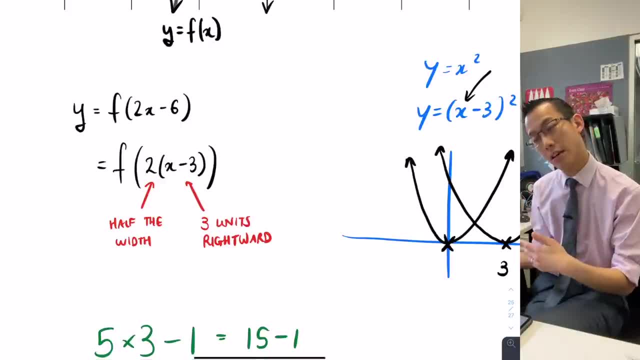 check it out. we've done half the width, Mm-hmm, Okay, And now we've got to do the other transformation, which is three units to the right, which in some ways is even easier than what we did just now, because you're like, oh, 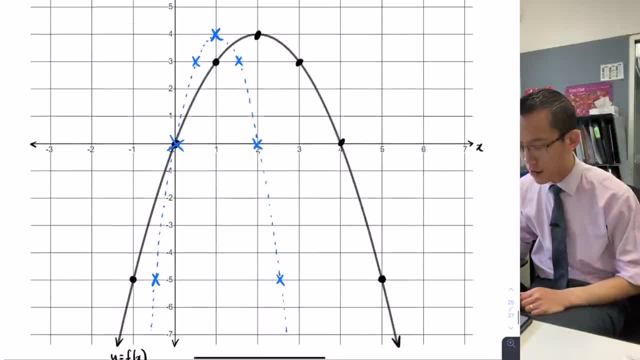 just everything, Just move, Yeah, just move it right. So it makes sense to take those same. what are we? how many do we get? We had five points, Yeah, Five points, And to move all of them, three units. okay, 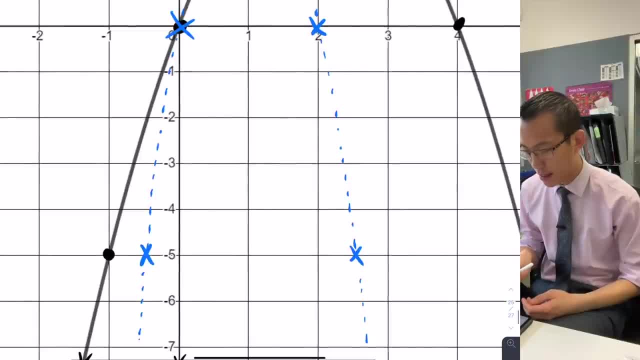 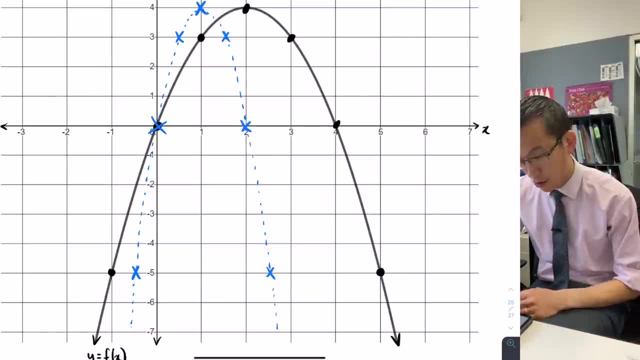 So let's just go from left to right. That first one you can see there on the left it's at negative a half. Yeah, So when you add three It just moves to like where that one is. Yeah, it moves to two and a half. 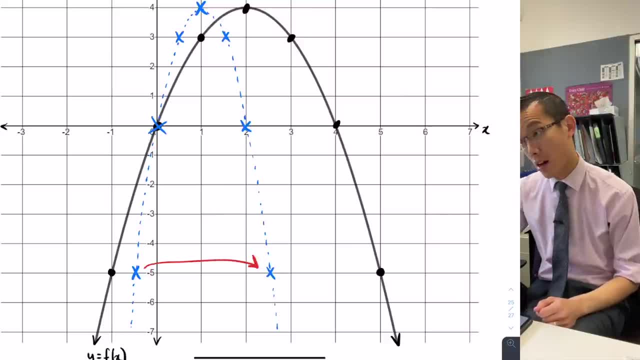 That's interesting. So I'm actually going to. you don't have to put this on yours, but I'm going to show in this other colour. Okay, Instead of using an X, because I don't want to confuse the stuff here, I guess I'll put a big fat dot. 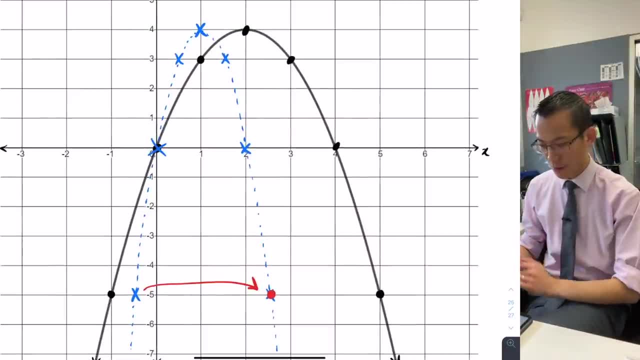 in red, okay, Mm-hmm, All right, Let's keep on going from left to right. So I've got that thing at the origin, right? Yeah, So it moves also three units, Everything goes. three units, So yeah. 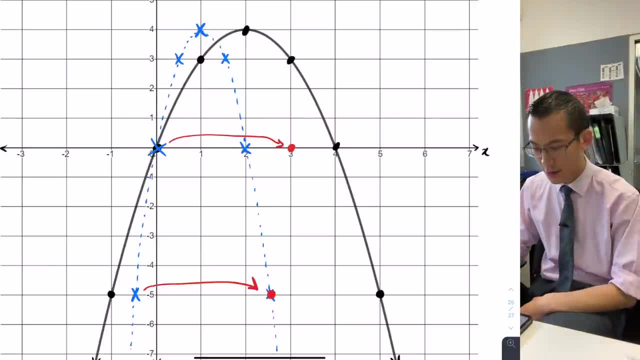 it's going to be moved over to three. You're going to keep going, right? You tell me what to do. next. You move the half to three and a half. Mm-hmm, Fantastic. So there we go. It moves over. 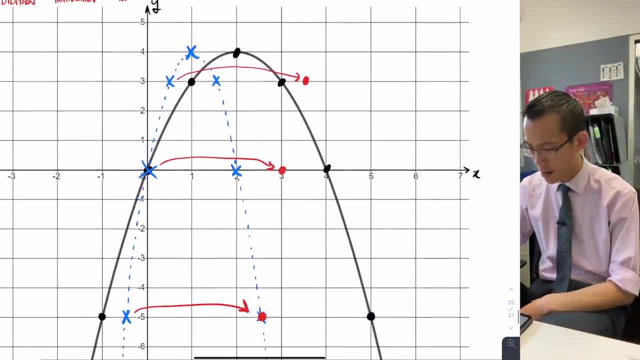 You move the stationary point to Four Yep, It was at one and now it's at four, Very good. And then you move at the other point, The next point, The next point, Sorry, just like The next blue point. 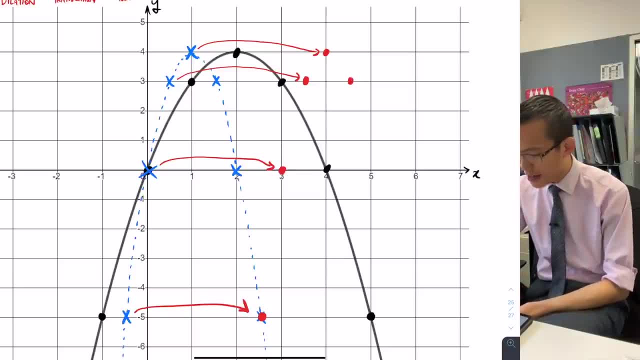 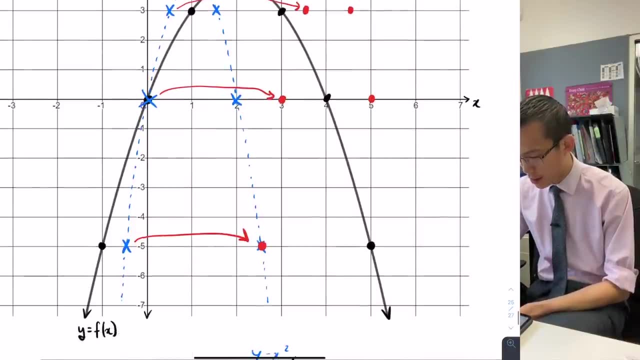 Yeah, from one and a half to four and a half, You're sort of getting the hang of this right. Yeah, In fact, you can kind of see the shape itself, just sort of following the pattern that you've already established. Yeah,